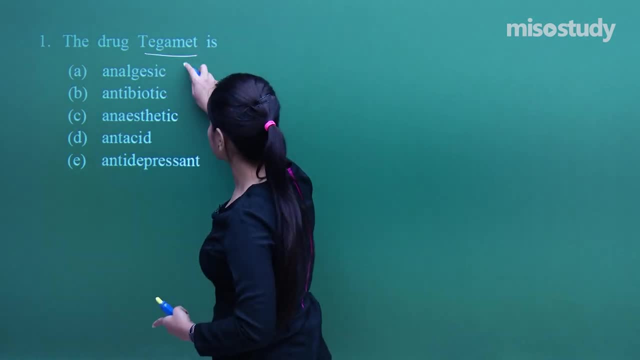 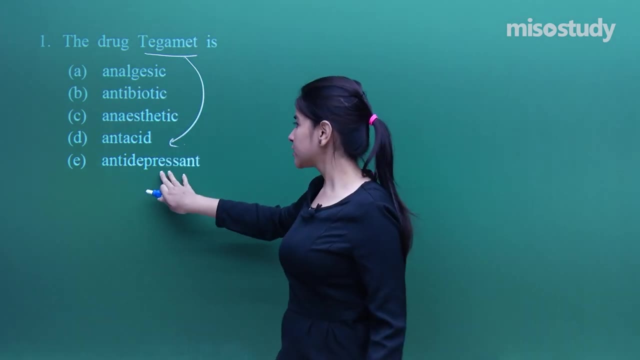 class of compound the Tegamet belongs to. So it belongs to the class of antacid, not analgesic, not antibiotic, not anesthetic, not antidepressant. And I would like to tell you here that J main pattern does not include the fifth option. But I have given I have included certain questions in. 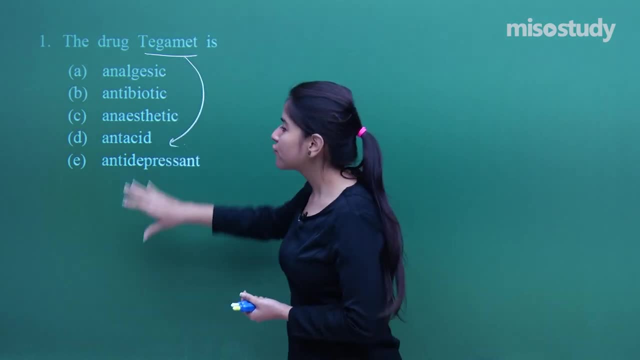 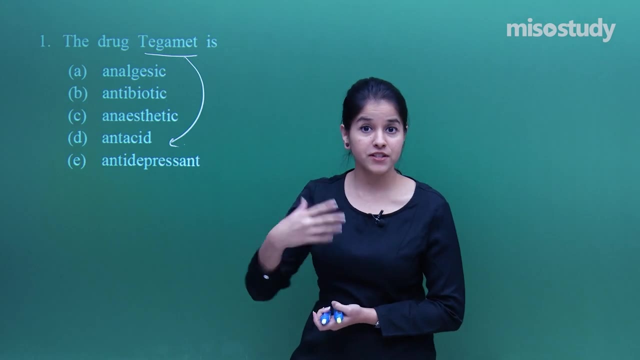 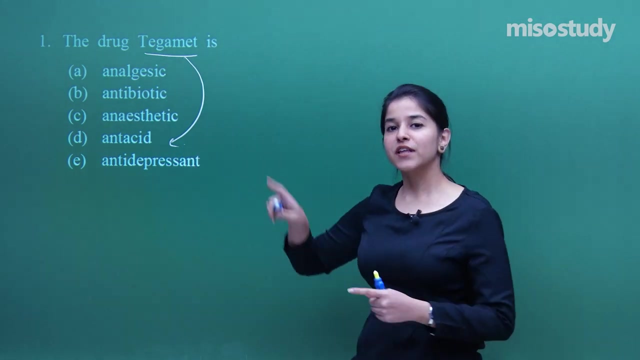 here in this questionnaire round, which actually has five options, So you be more careful, so you will have to choose out of five. now the difficulty level has increased, So let us just try to test your knowledge. So the drug Tegamet is an antacid, So that is the actually common 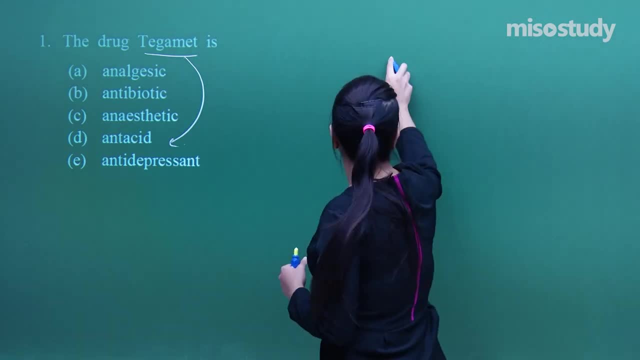 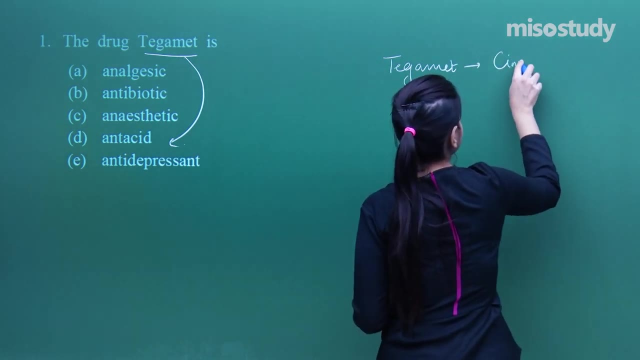 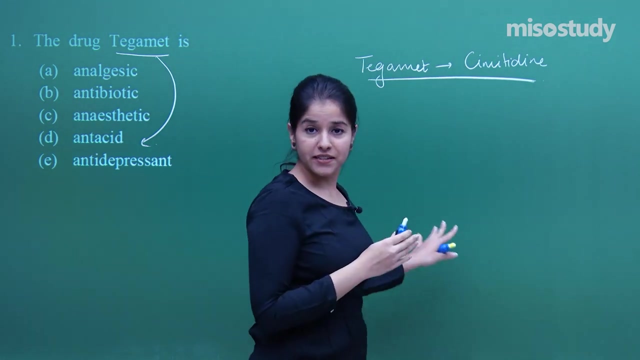 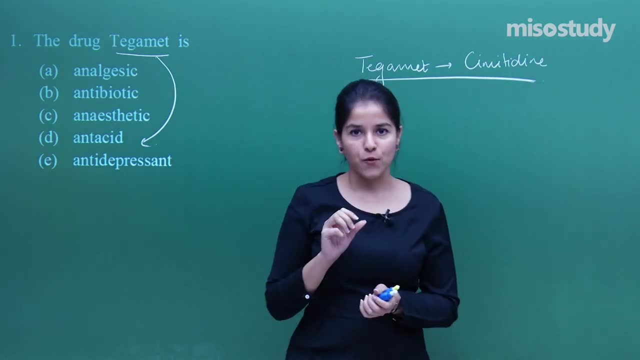 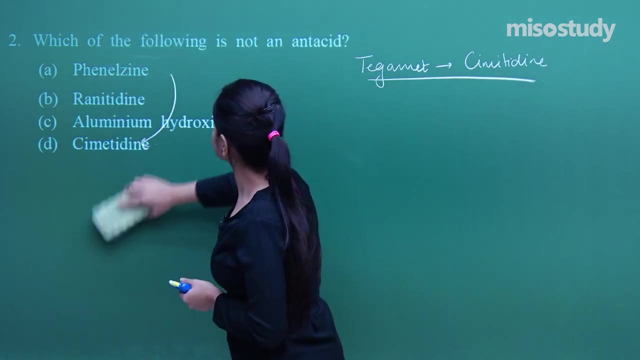 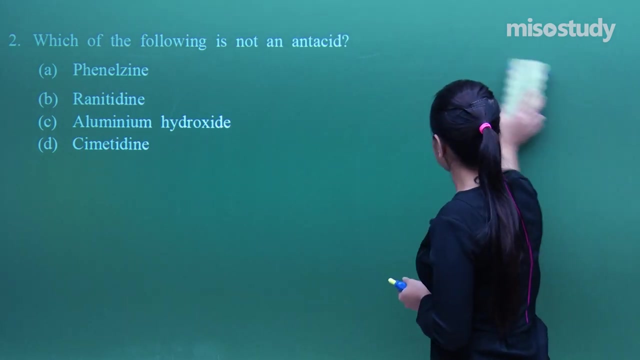 I hope everybody is clear with the concept. Now let us move on to the next question. What do we have here Now? it says which of the following is not an antacid, So I need to have the one which is not. So be very. 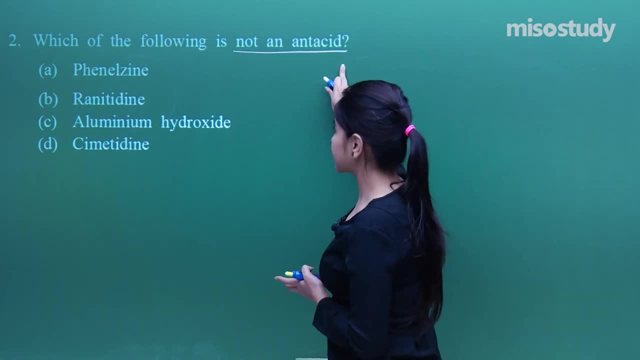 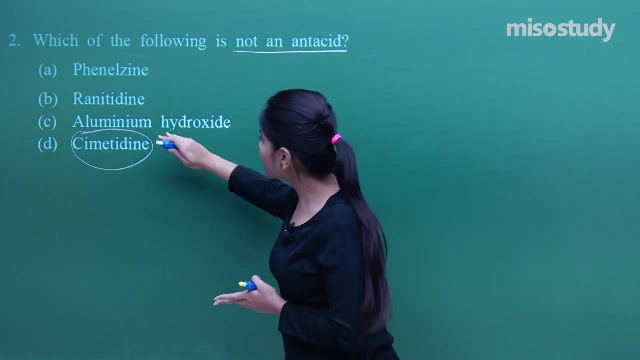 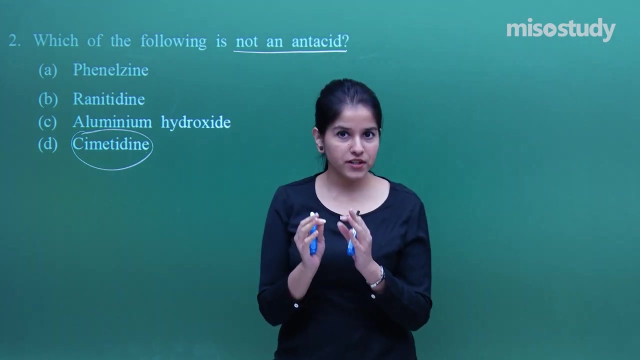 careful while reading the question. Not an antacid, That means we already have done done that. Cimetidine Is an antacid. If you look over here- aluminium hydroxide- and try to recall the concept of antacids, Antacids are actually the drugs which are necessary whenever we have got acid production- more of acid production- in our stomachs during the digestion process. 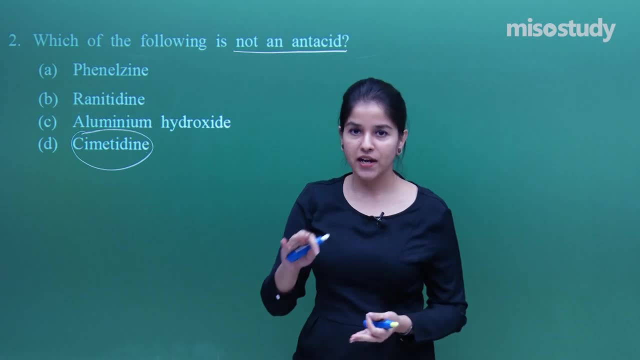 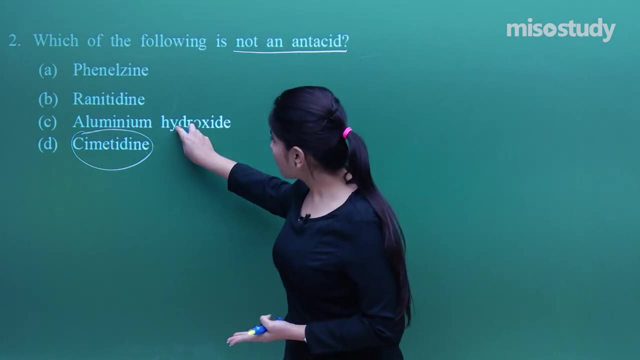 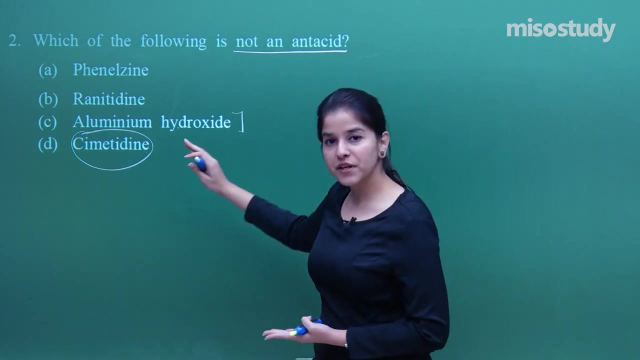 So that could hurt our stomach. In order to neutralize that acid, we can use weak bases as the neutralization chemical. So in that category I can also apply aluminium hydroxide for that use. So aluminium hydroxide is a weak base. It can be used as an antacid. So that is also not the case. 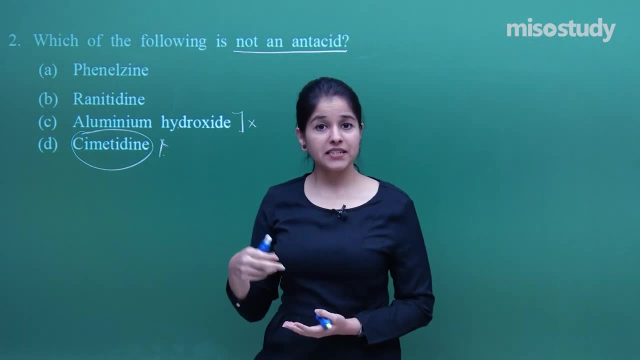 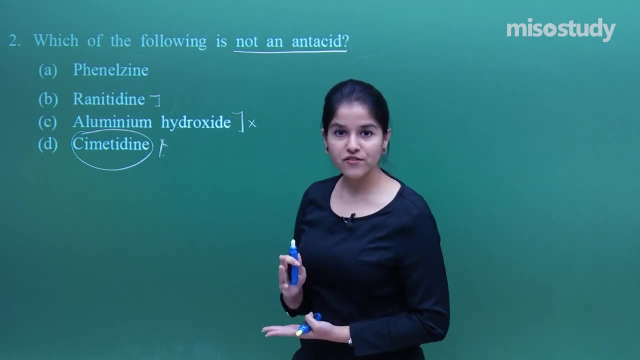 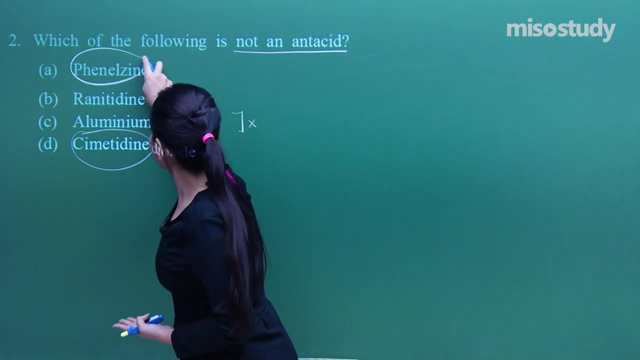 Now comes the ranitidine. What is ranitidine? It is very widely used, Or we can say a revolutionary antacid that was made. So, again, ranitidine is also an antacid. not our option We are left with is phenylzine, which is not an antacid, and that is our answer. What is phenylzine actually? 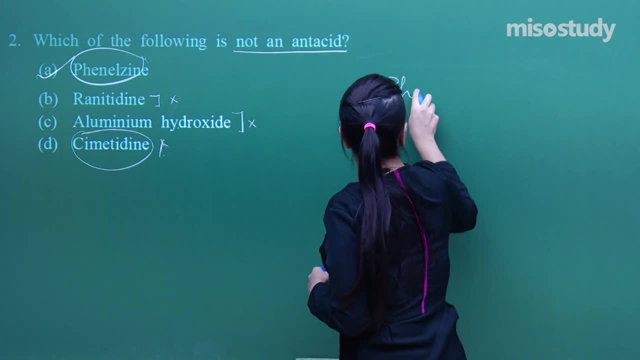 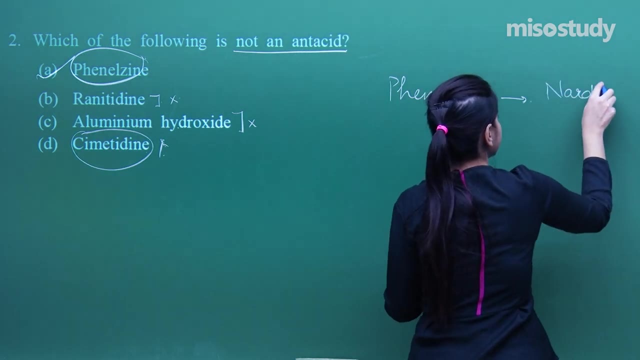 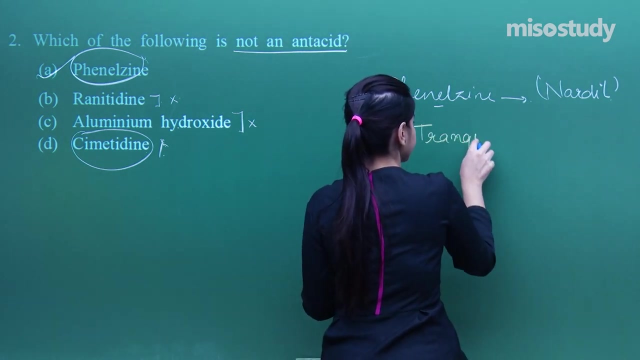 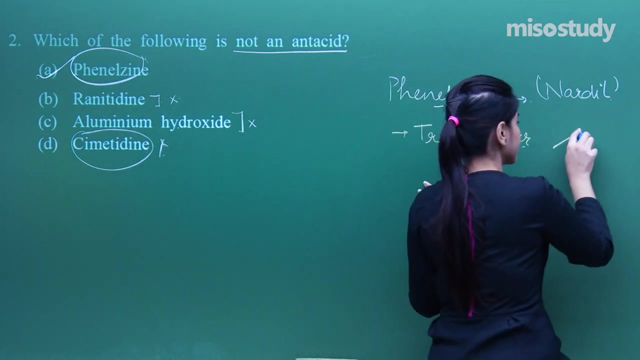 If you are able to recall it, phenylzine is also known as nardyl. It is a kind of a tranquilizer. So that is tranquilizer, or I can say it is antidepressant. So what is the formula for it? Phenylzine is like this. 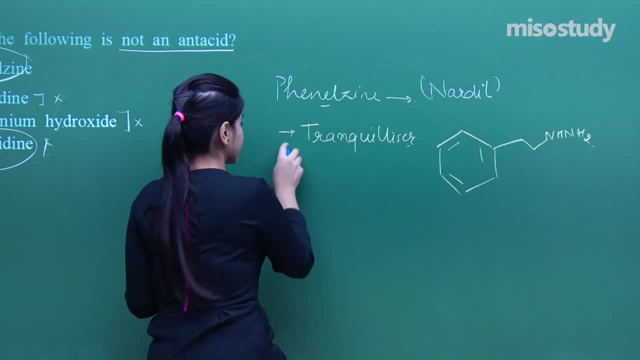 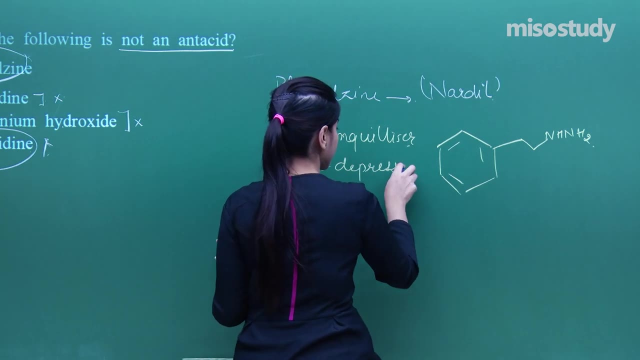 So that is what. phenylzine is also an antidepressant, So I hope everybody knows. So that is what phenylzine is also an antidepressant, So that is how to draw the structure: Antidepressant. 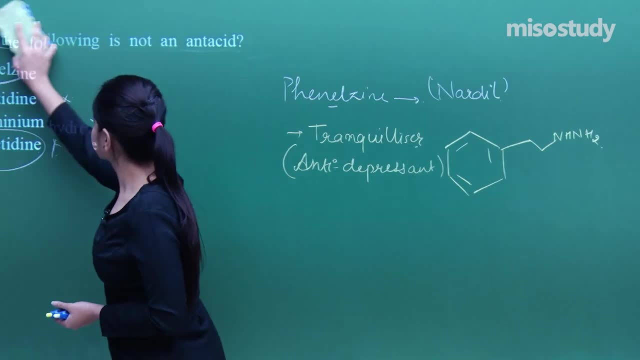 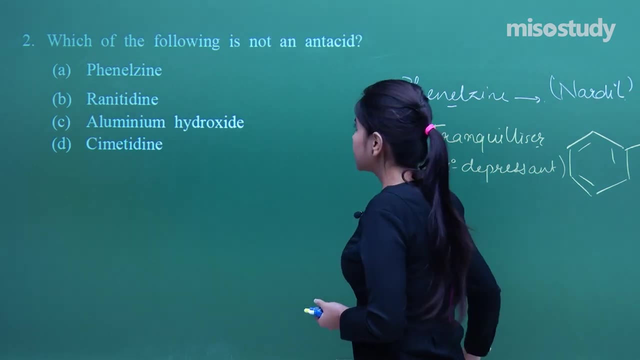 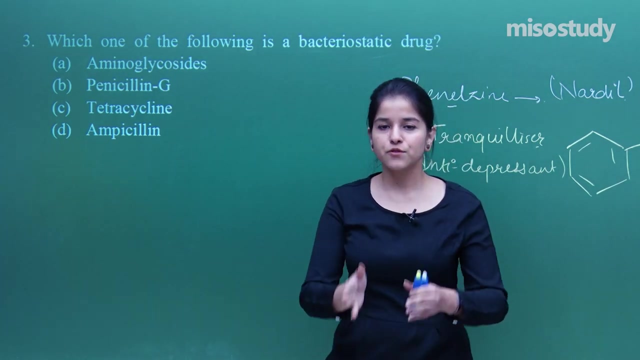 Now let's move on to the next question. So these are pretty simple questions. You just need to recall the concept and what all structures we have got Now. which of the following is a bacteriostatic drug? So we have learned: in the category of antibiotics we have got bacteriostatic as well as bactericidal. 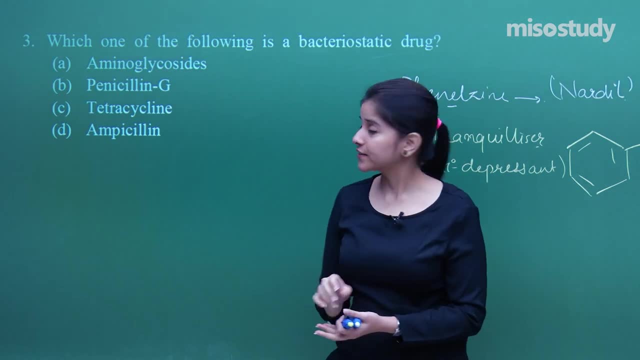 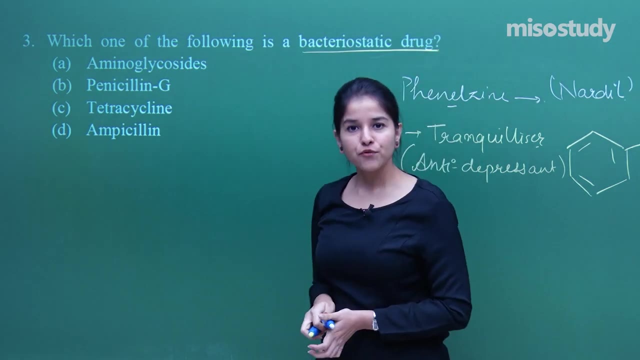 Bacteriostatic are the ones which stop the growth of microorganisms. So out of all, I need to find out those which are bacteriostatic drug. So we have learned what is aminoglycosides. 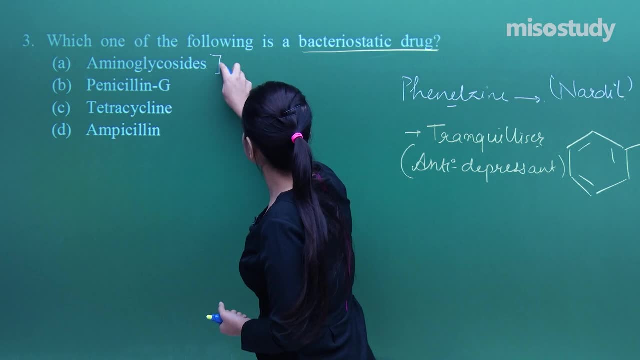 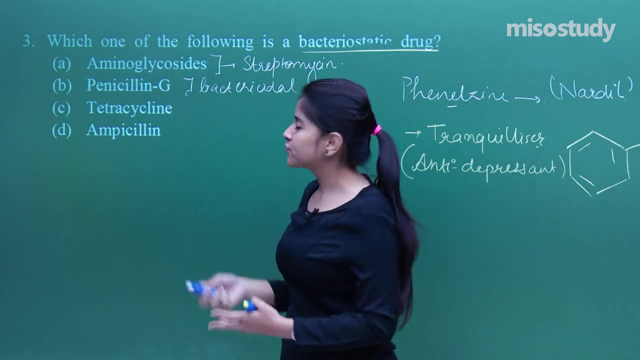 Again, it is bactericidal. So that is bactericidal. Nothing but streptomycin In the case of penicillin G. so it is a worldwide used antibiotic, Also bactericidal, So included under the category of bactericidal tetracycline, and we are left with ampicillin. 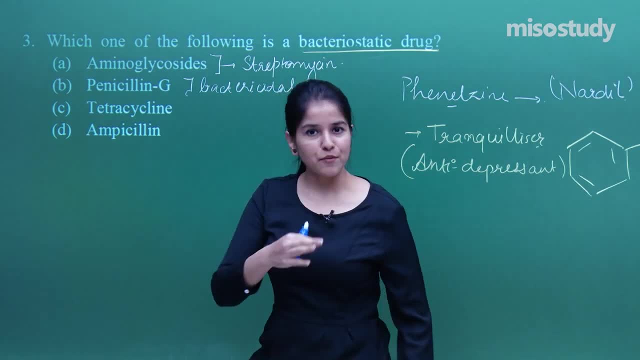 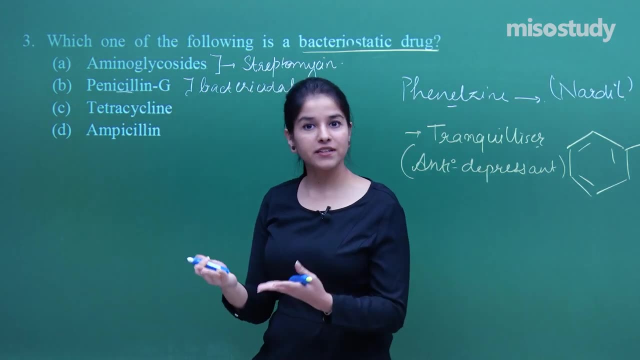 So I would like to discuss here what ampicillin is. It is a semi-synthetic modification of what we have in penicillin, So the penicillin is modified into another kind of a drug, that is, ampicillin. 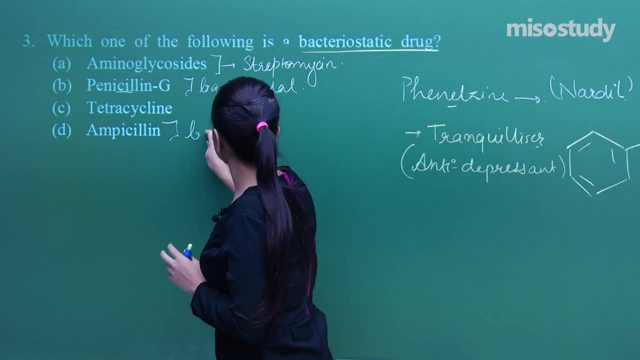 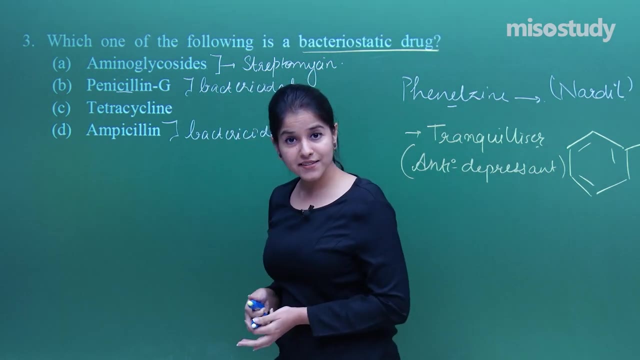 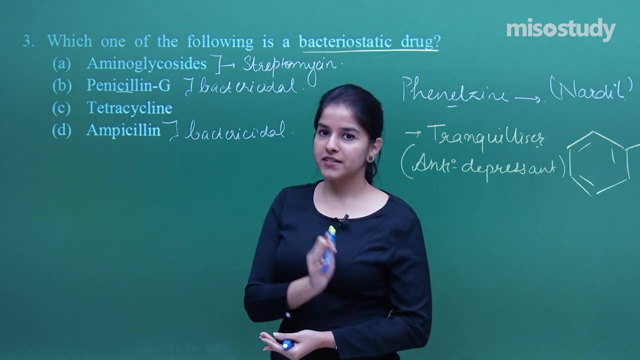 Again, what Bactericidal. So that is also bactericidal. So I hope everybody has got the answer. that is tetracycline Here. in this case it stops the growth of microorganisms. Being an antibiotic, it is not killing the bacterias, but stopping its further growth. 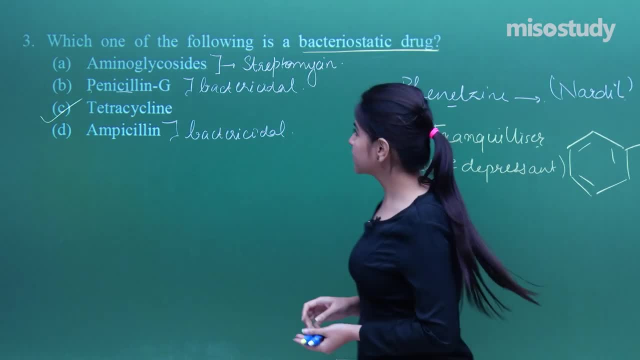 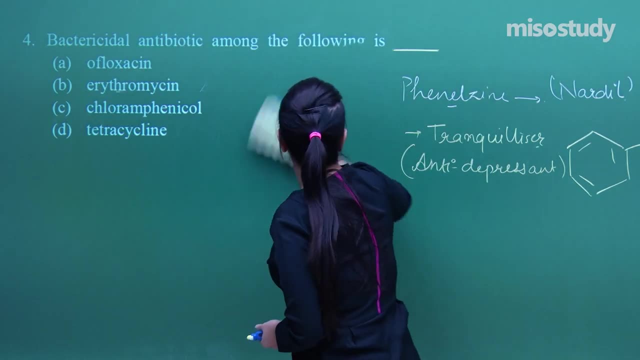 So I hope that is very well clear to you and you have got the right option. Now let's move on to the next very question: What do I have? Let me just rub this off first. Okay now. Now they are asking: 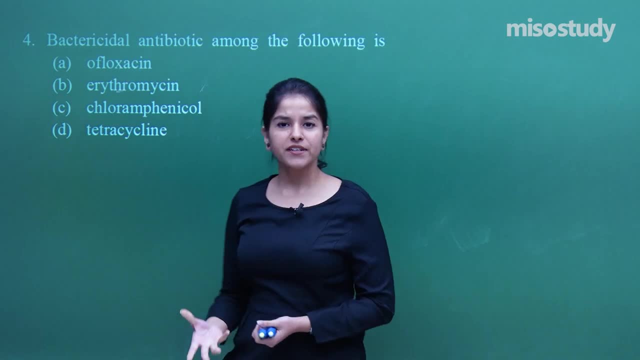 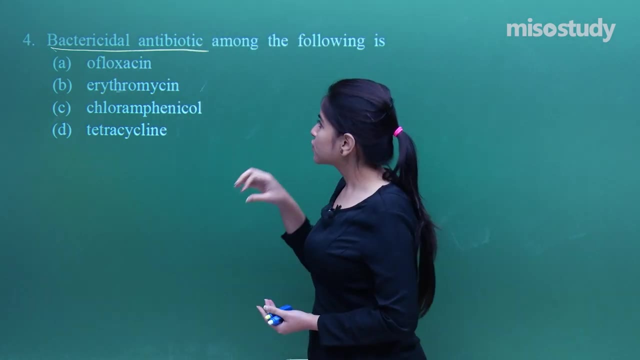 Bactericidal antibiotic. So we have already discussed that. Let us just mark out our correct option. So I need to have the bactericidal antibiotic. One is ofloxazine, erythromycin, chloramphenicol, tetracycline. 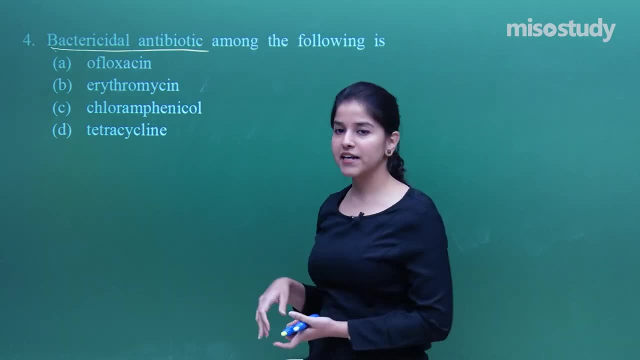 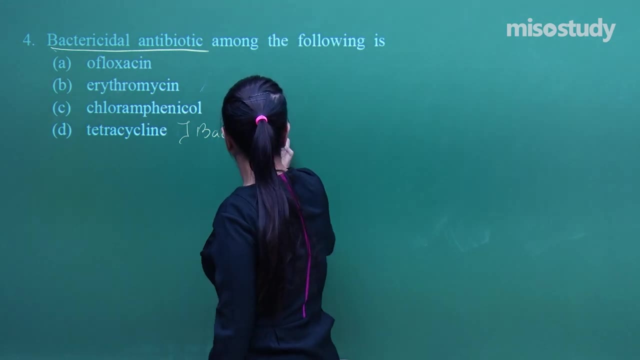 So we have already done. Tetracycline comes under the category of bacteriostatic, So that is bacteriostatic. Now comes the chloramphenicol, So that is bacteriostatic. Now comes the chloramphenicol. 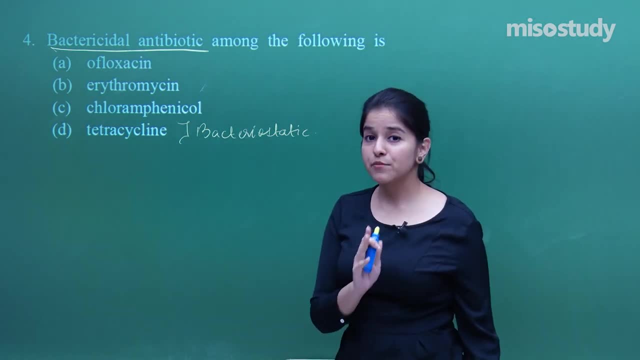 You can call very, very popular medicine very, very popular antibiotic. Why? Because it is a broad spectrum antibiotic. It covers a range of microorganisms. It kills a range of microorganisms. So that is what It is not killing, but stopping. 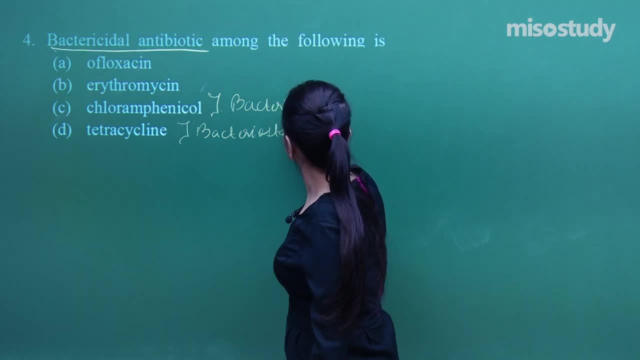 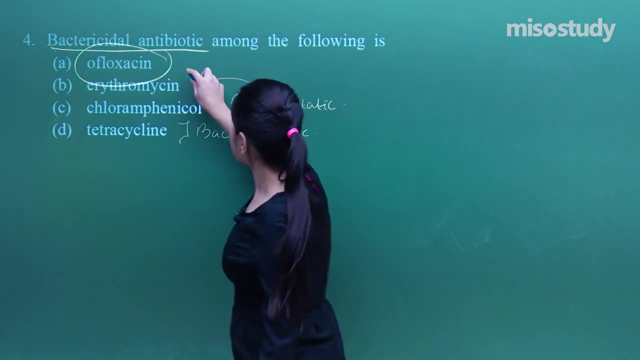 Again, it is bacteriostatic. What comes next? Erythromycin- Again a bacteriostatic. Now we are left with is ofloxazine. I hope everybody is clear with the concept. This is bactericidal. 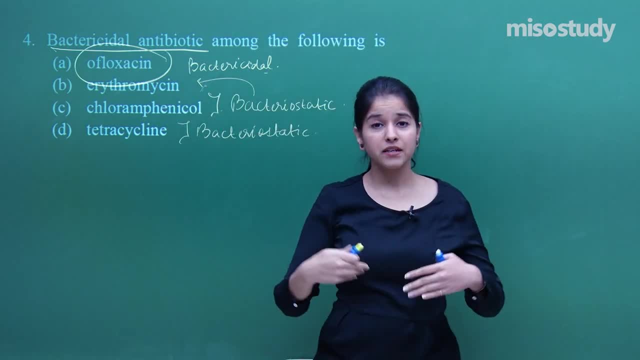 And in the case of some kind of infections, or you can say, broad range of infections, ofloxazine is always preferred. You might have observed a doctor prescribing you oflox, something kind of a medicine That is nothing but containing the drug ofloxazine. 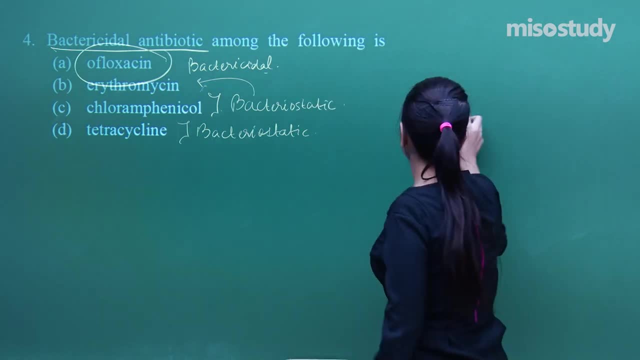 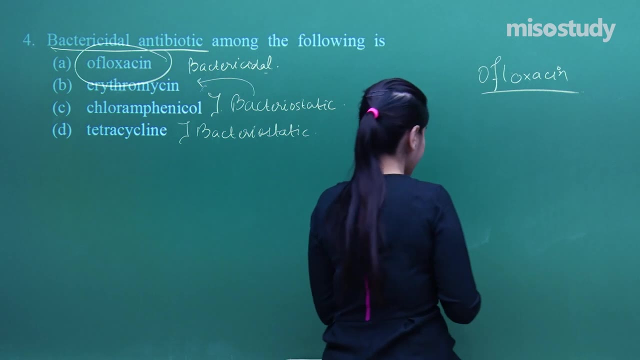 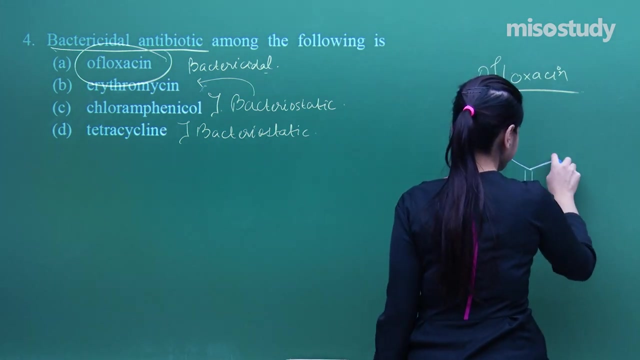 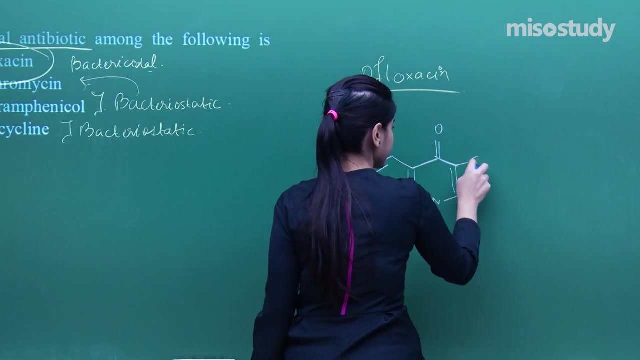 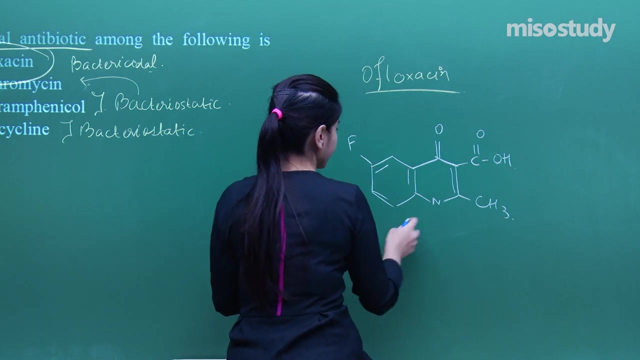 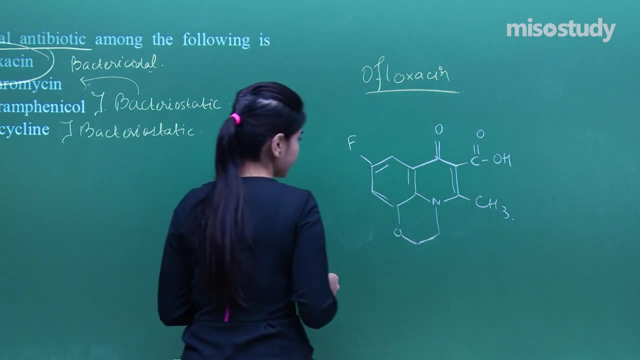 I hope everybody is clear with that. So let us just draw the structure of ofloxazine: Ofloxazine. The structure is somewhat like this, So I hope everybody is able to make it, And yet it is remaining. 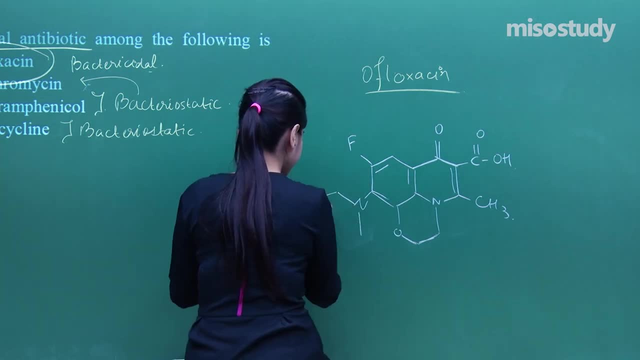 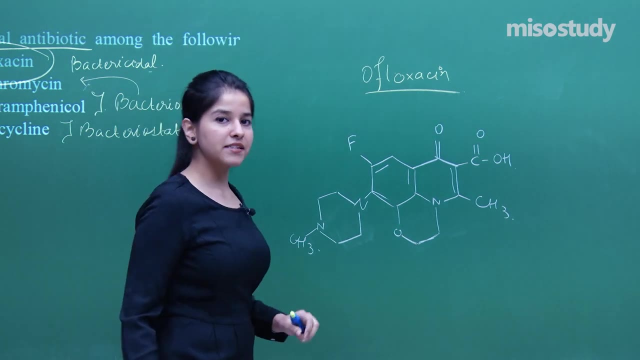 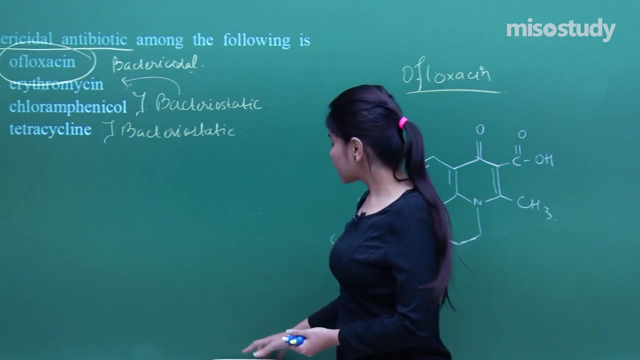 So that is what its structure is. This is nothing but the ofloxazine. I hope everybody is clear with that And you have got this structure right, I hope. Now let us move on to the next question. 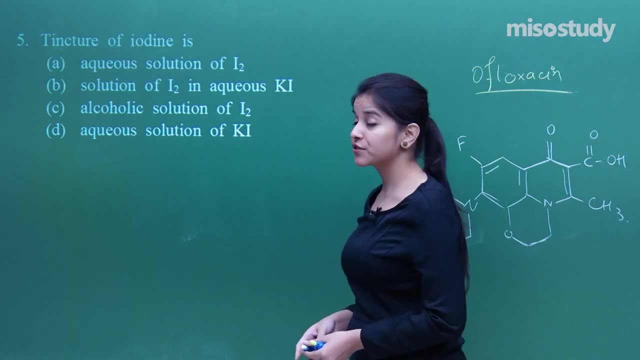 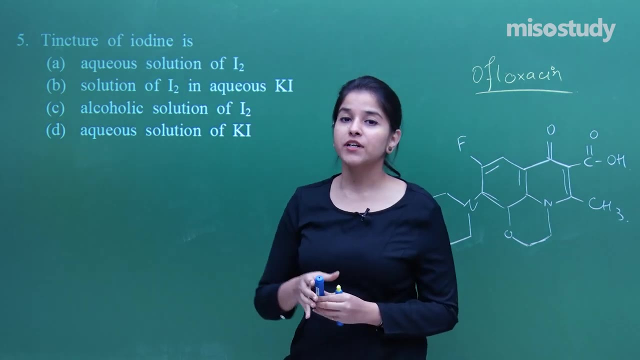 So the next question says: tincture of iodine is. So it is a very, very important question you can say, Because tincture of iodine is most prominently used: What kind of drug is that That is antiseptic? 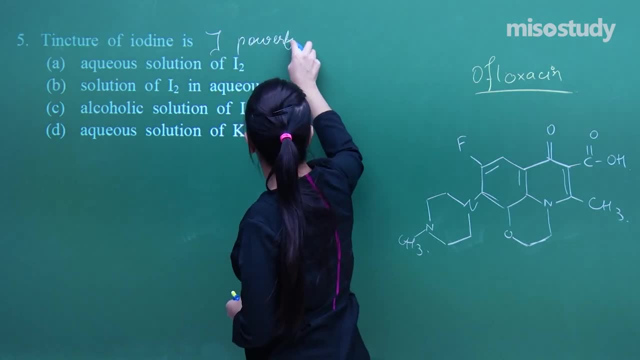 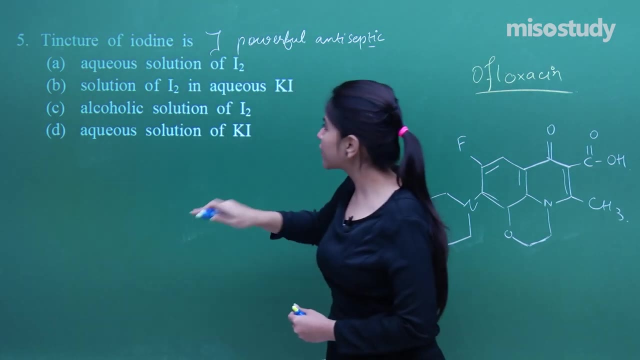 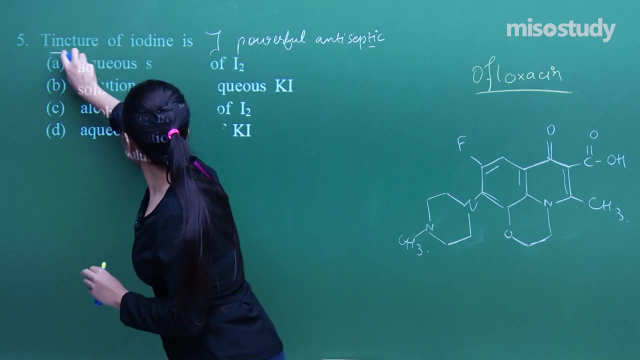 So it is a powerful antiseptic. So, as the name suggests, it contains iodine. So each and every option is actually having iodine in it. But what is the specification for the formation of tincture of iodine? 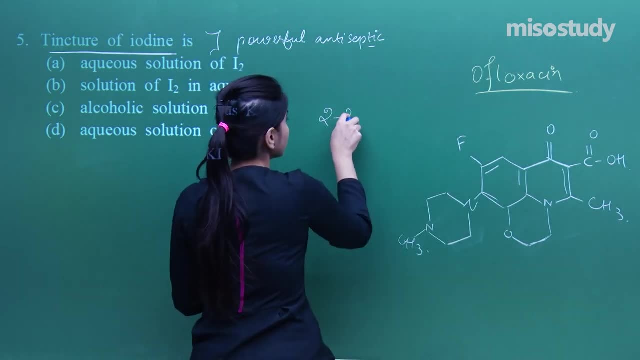 I hope you all know the specifications. It is 2 to 3 percent I2 solution in C2H5OH. that is the alcohol And water. So that is what the specification in the case of tincture of iodine is. 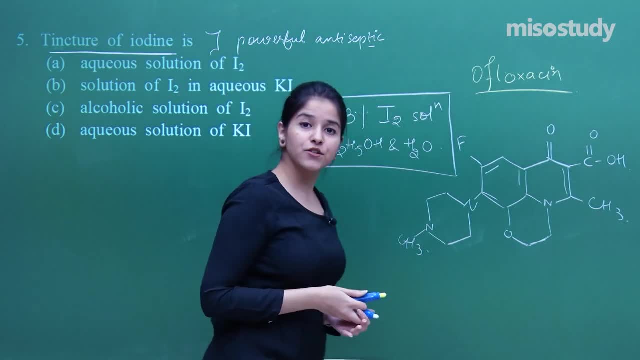 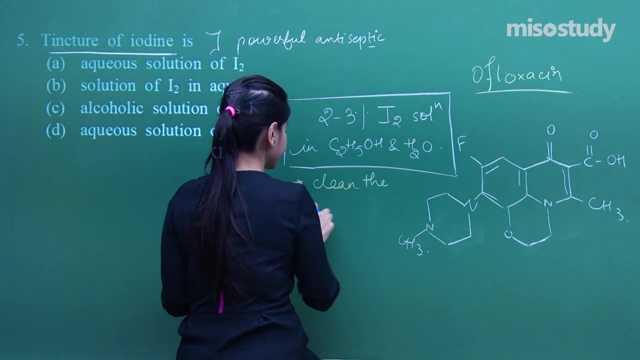 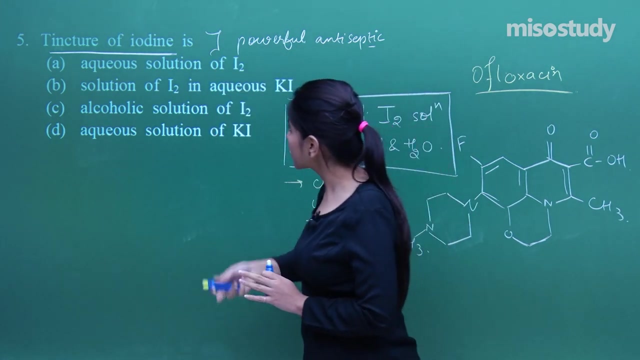 And it is a very popular antiseptic. Where is it used? It is used to clean the wounds. So it is used to clean the wounds. So now we are through with the question. Let us just mark out the answer, the correct answer. 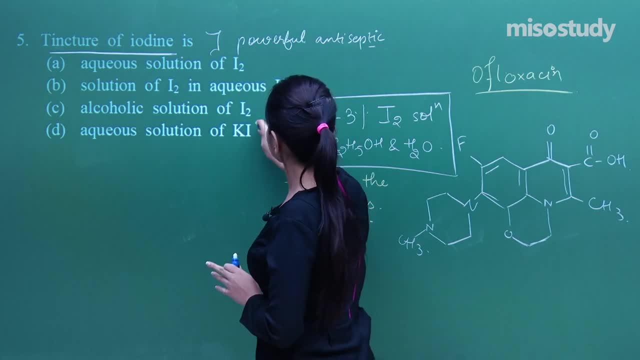 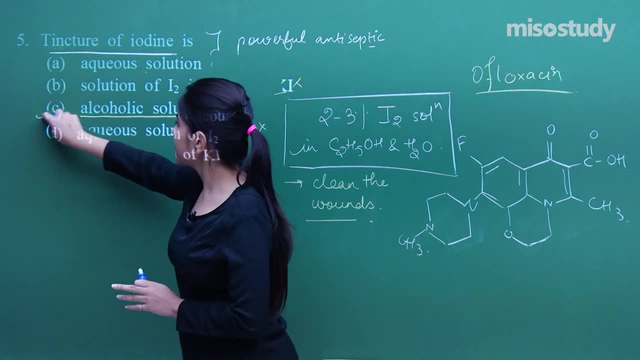 So it is the alcoholic solution of I2, not Ki. We are not concerned with the Ki, Not just the aqueous solution of I2,, but containing alcohol. So alcoholic solution of I2 is the right answer. So let us move on to the next question. 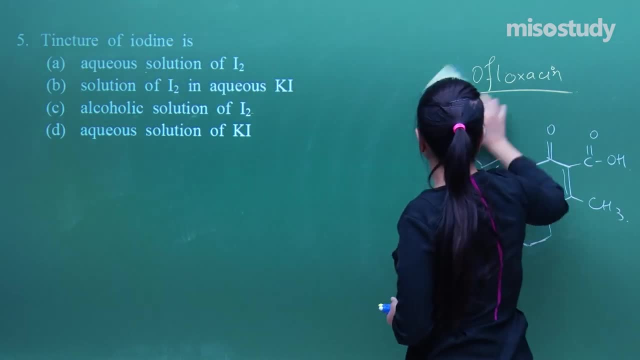 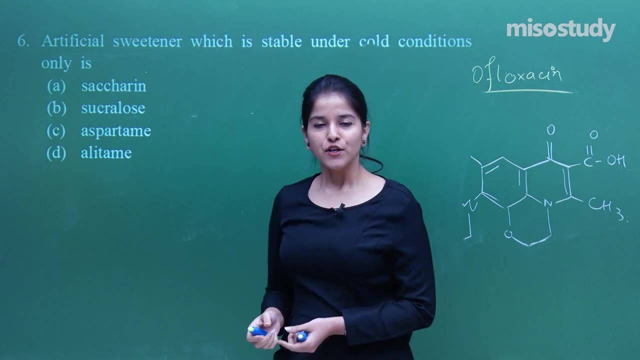 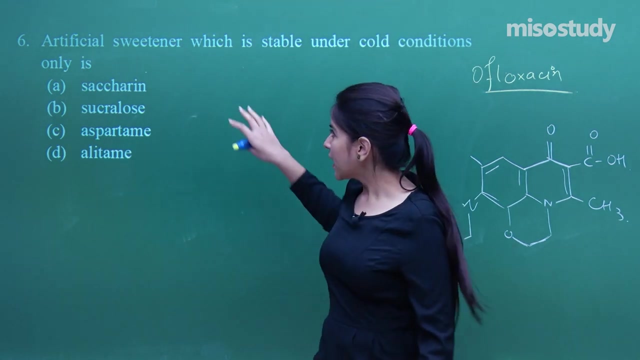 So the next question says artificial sweetener which is stable under the cold conditions. So you must be having a very, very good knowledge of the artificial sweetness. Almost each and every time, at least one question is expected from this very topic. 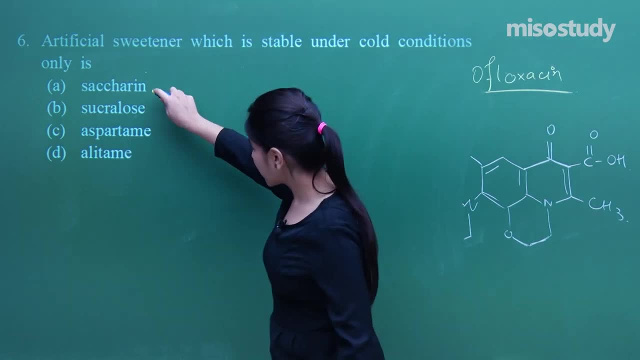 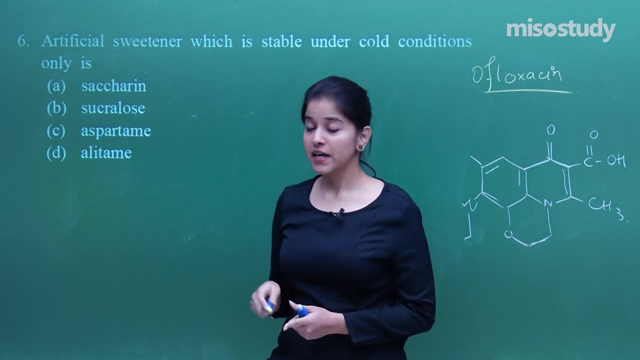 So artificial sweetener: I have got saccharine, I have got sucralose, aspartame, alletame. So if you all know that alletame is what Alletame is actually the highest possible sweetener. 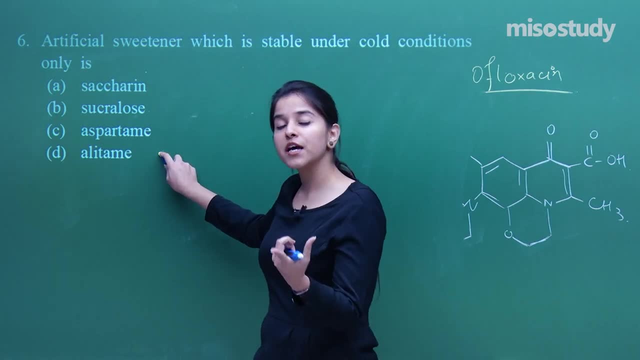 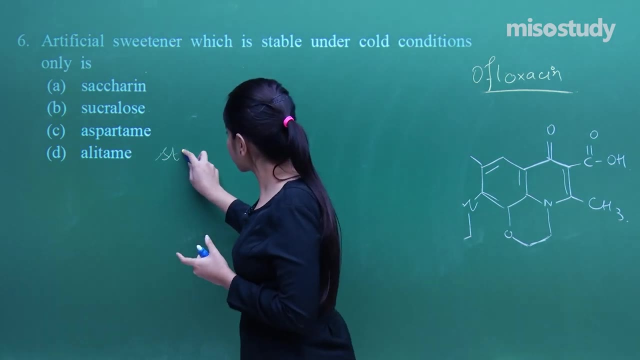 That is approximately 2000 times sweeter than sucrose And it is also stable at higher temperatures. So it is stable at high temperatures. So that is stable at high temperatures. Also, what Aspartame, sucralose and saccharine? 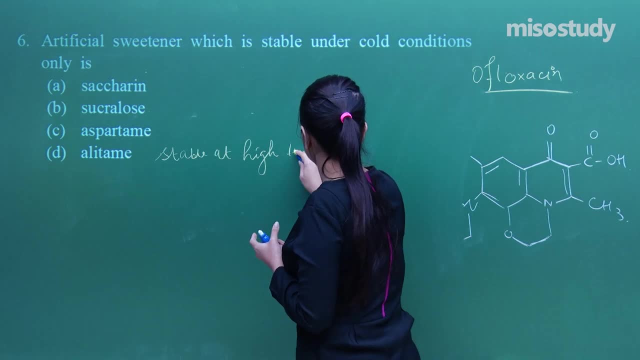 So we all know what saccharine is. Saccharine is actually 550 times sweeter than sucrose And it is most prominently used, but it again sustains temperature. If I talk about sucralose, then I say that it is more than that. 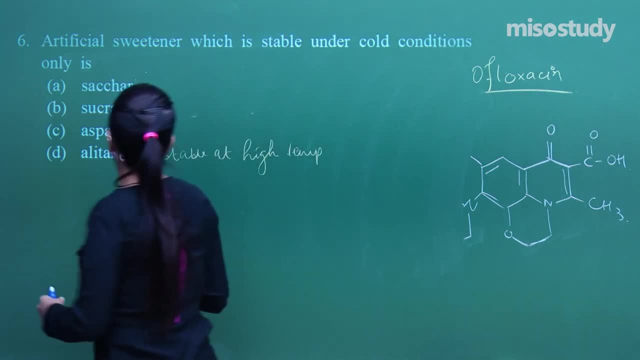 That is why I have taken the one that is more than that. So that is why I have taken the one that is more than that And it has more than that. So what else? So, it has more than that. 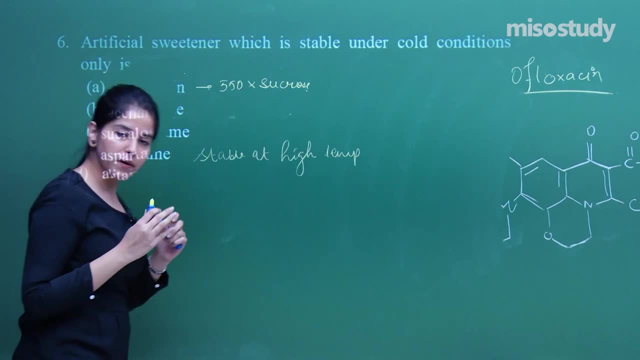 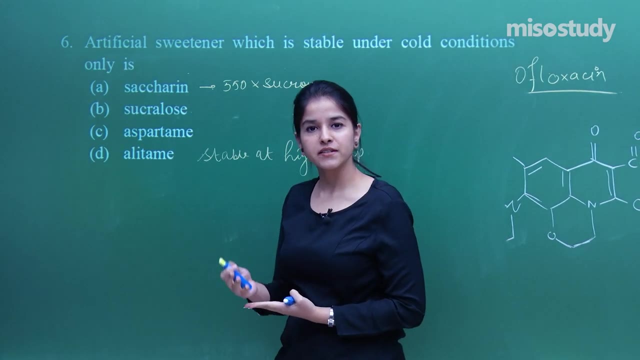 So it has more than that. So what else? If I talk about sucralose, sucralose again, it sustains temperature. it is mostly used for the baking purposes, for the cooking or baking purposes. 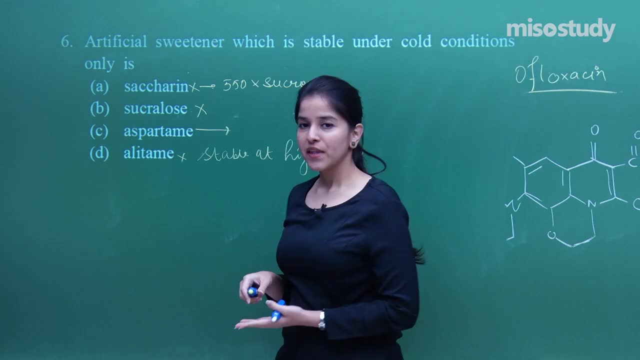 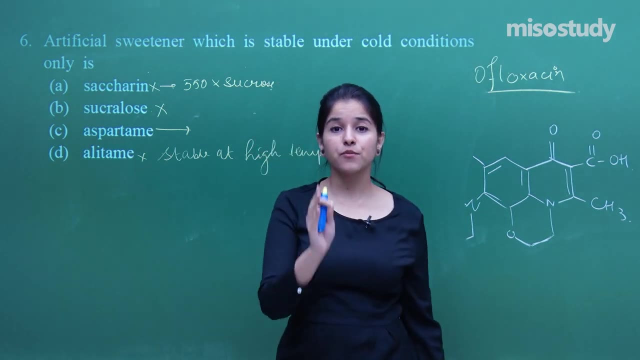 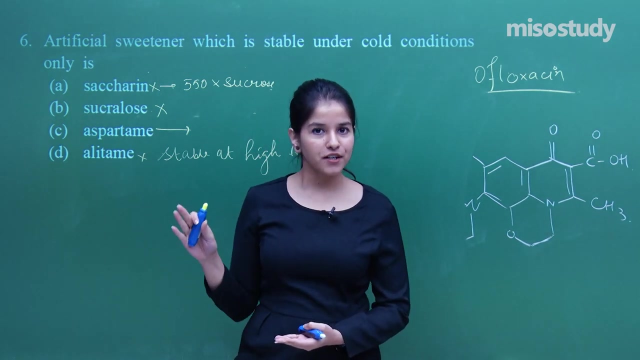 So these options are not included, but aspartame. Aspartame is most prominently used. If you have recalled the concept aspartame, the most prominent use, the most important use of aspartame is in the cold drinks Because at higher temperature it gets decomposed. 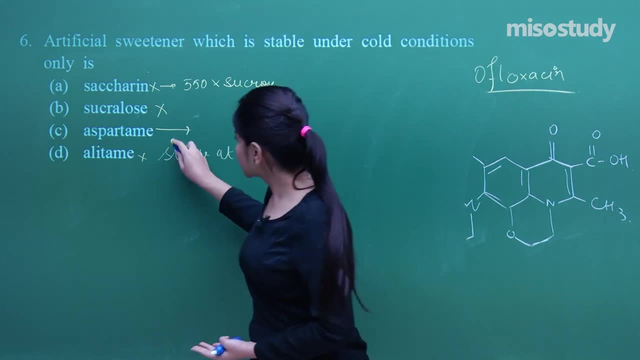 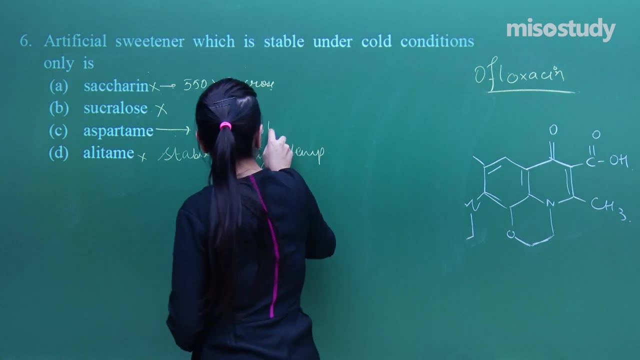 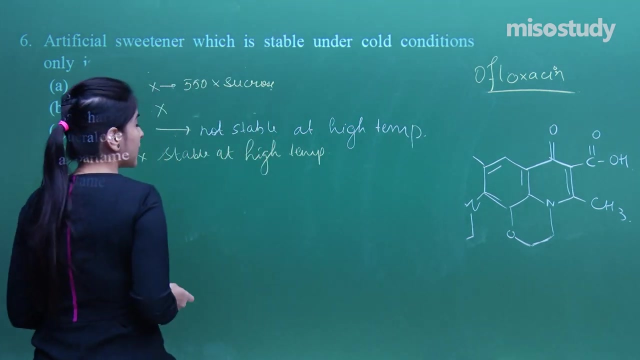 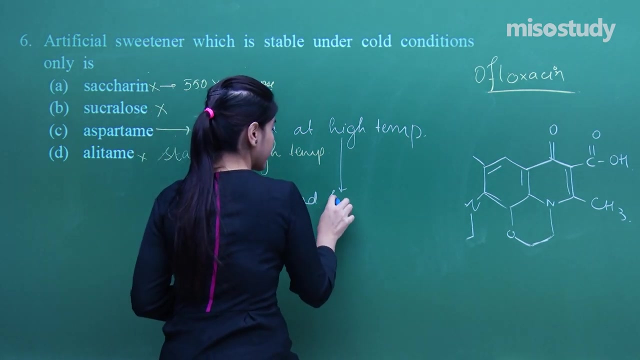 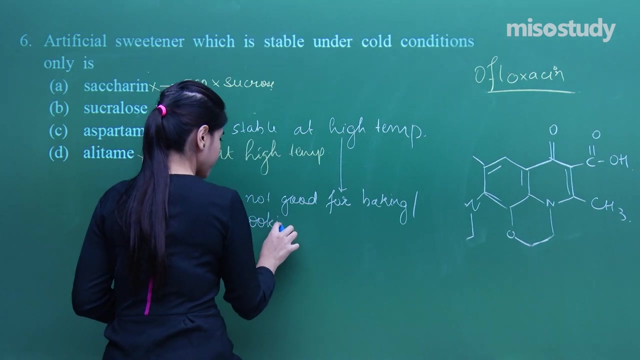 So it cannot be used in baking or cooking purposes. So basically, aspartame is not stable at high temperatures. That means what It is not good for baking Or cooking. Also, it decomposes at higher temperatures, So it is used in cold drinks. 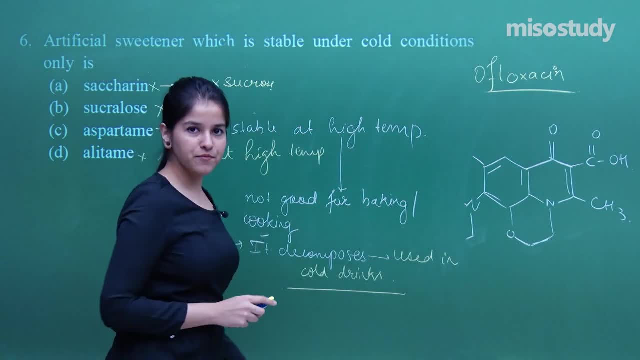 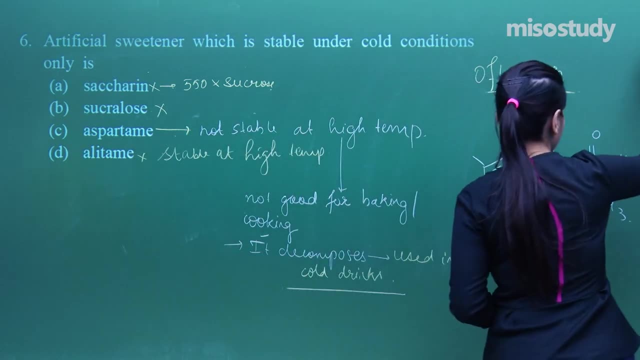 Now, what is the structure for aspartame? It is related to aspartic acid as well as the mycelium Methyl ester of phenylalanine. So what we have got in the case of aspartame. 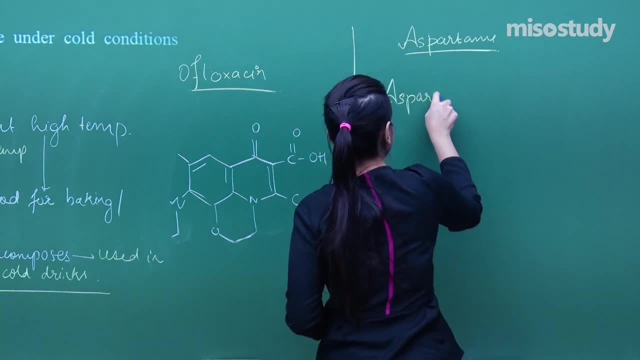 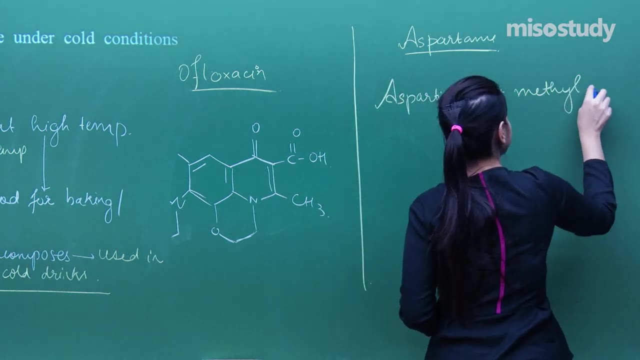 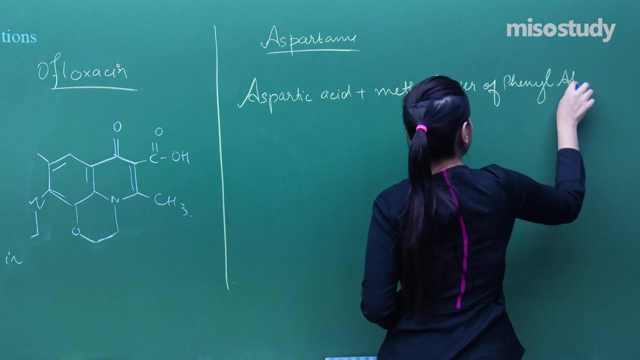 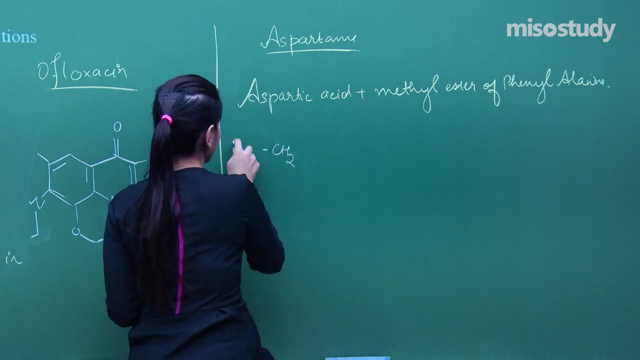 We have got the aspartic acid plus methyl ester of phenylalanine. Methyl ester of phenylalanine. Now, what is aspartic acid? It would be. CH2CWH is the R group, And what else do we have? 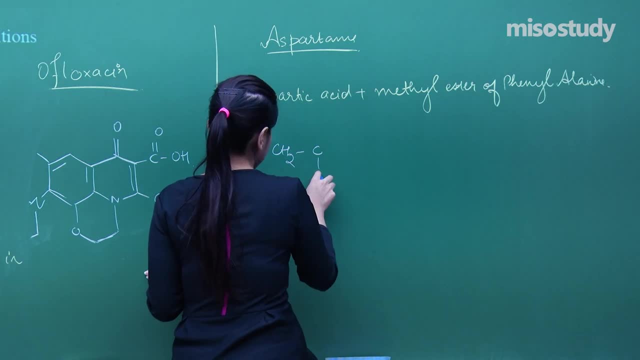 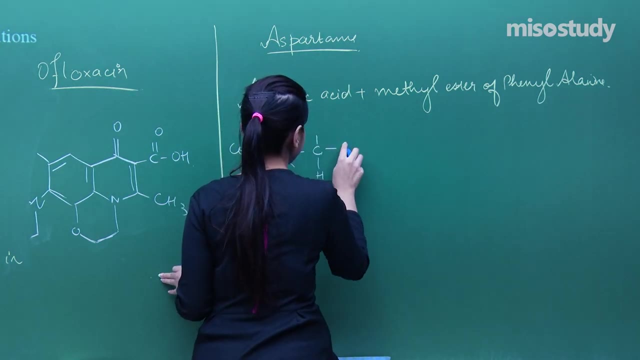 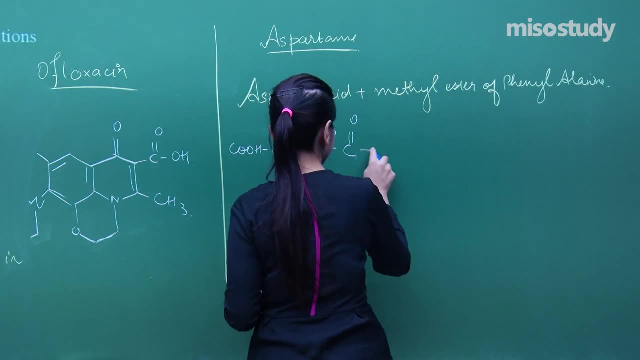 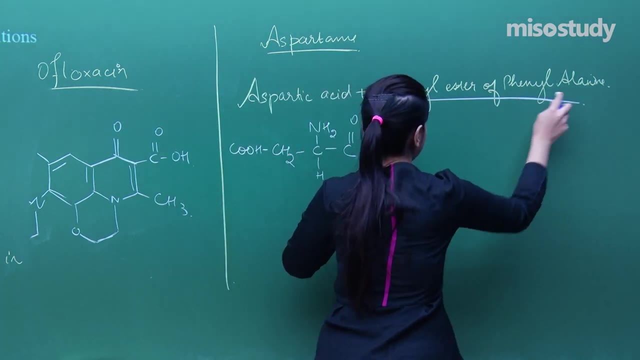 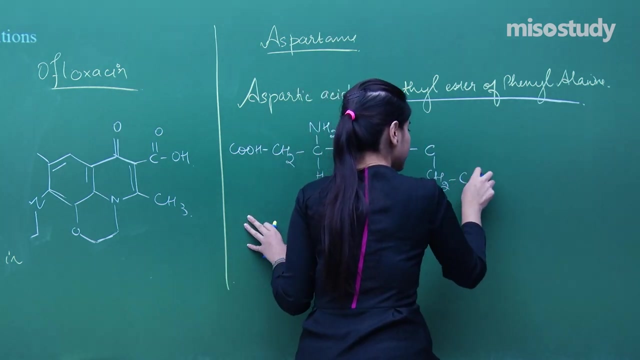 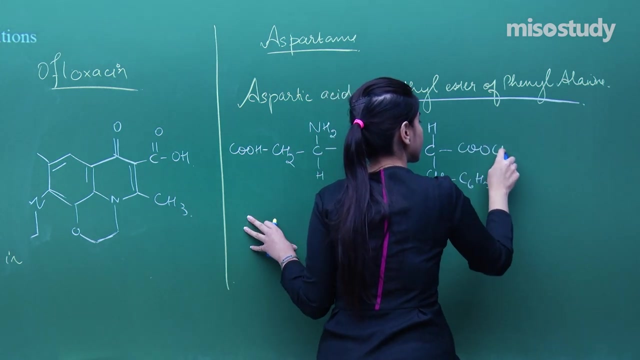 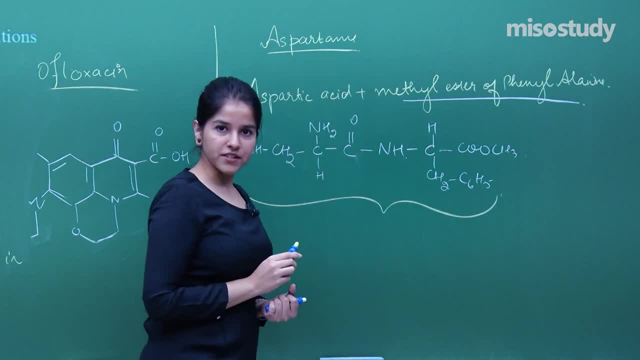 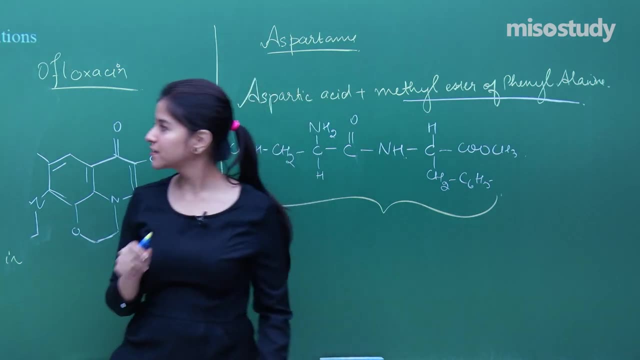 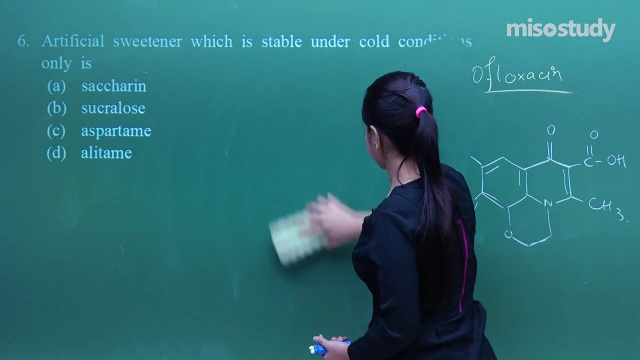 is the compound we need. This is aspartame and it is stable only at lower temperatures. that is used in the cold drinks. So I hope everybody is clear with the fact. Now let's move on to the next question. What do I have next? Salts of sorbic acid and propionic acid. 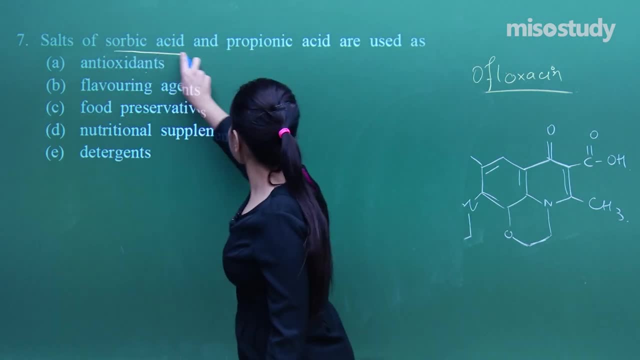 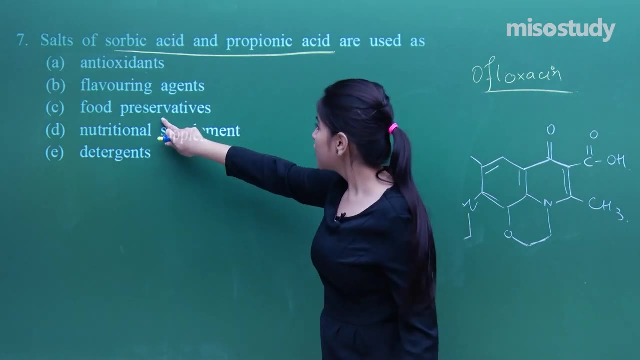 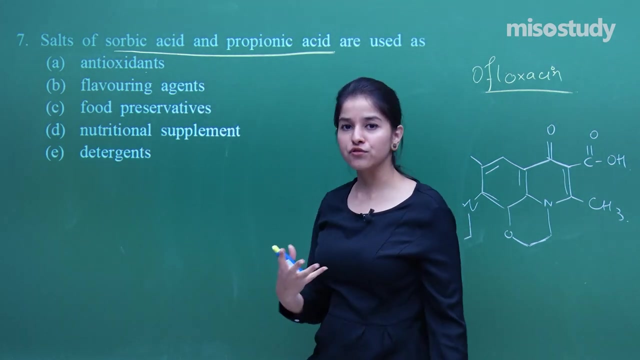 completely a factual question. So salts of sorbic and propionic acid: are they used as preservatives, antioxidants, flavoring agents? Again, 5 options here: Food preservatives, nutritional supplement and detergents. So if you try to recall all the kinds of salts, 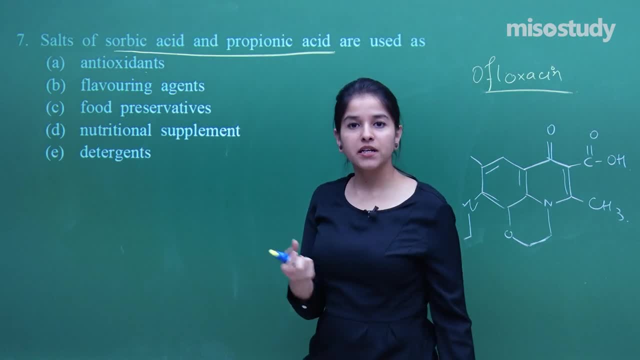 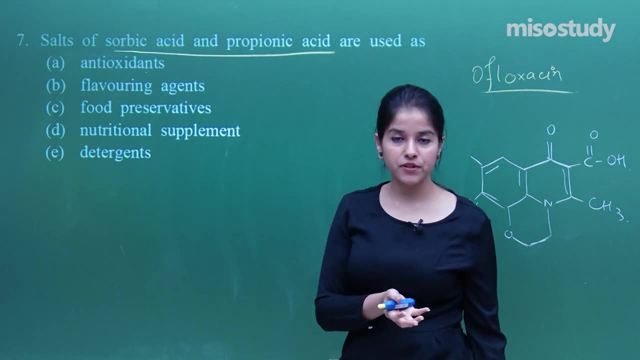 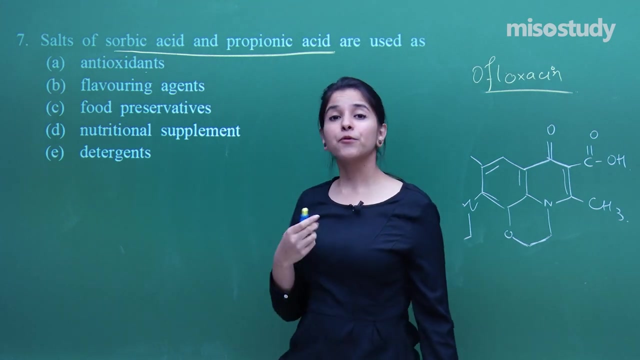 So those are actually just as what we discussed as the table salt. So table salt is used as a preservative. Sugar can be used as a preservative. These are the natural preservatives class 1 type, But if I talk about the class 2 types I get sorbic acid and propionic acid. 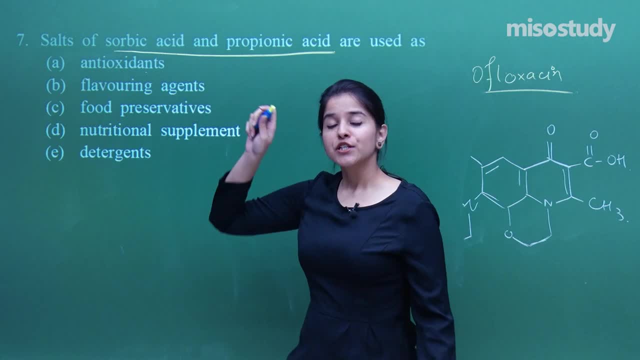 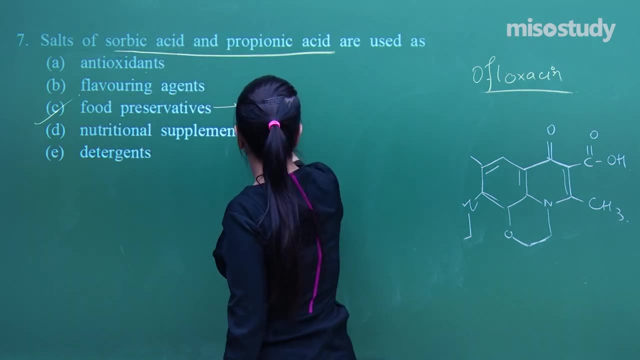 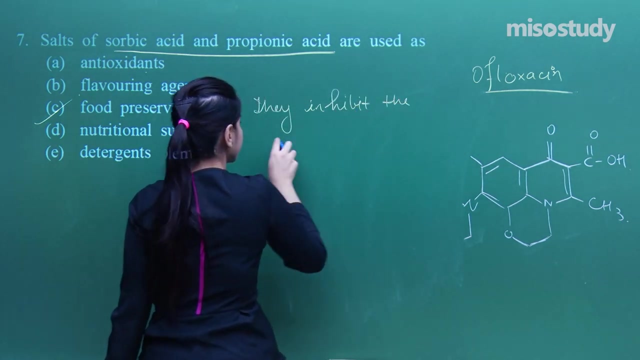 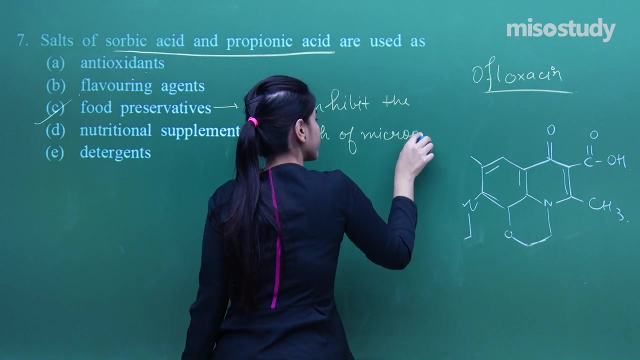 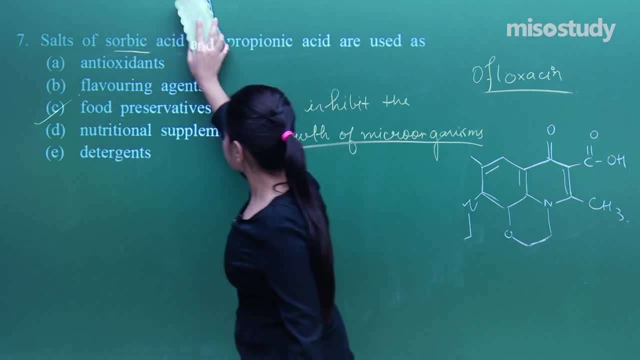 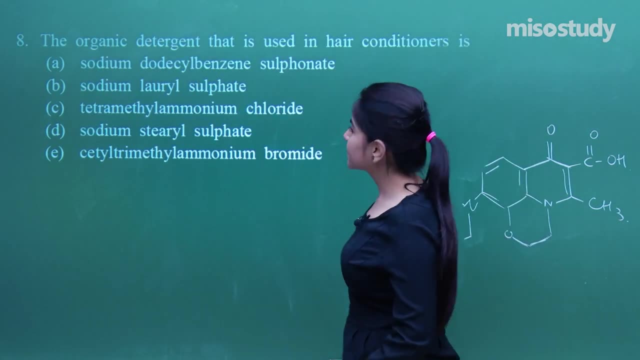 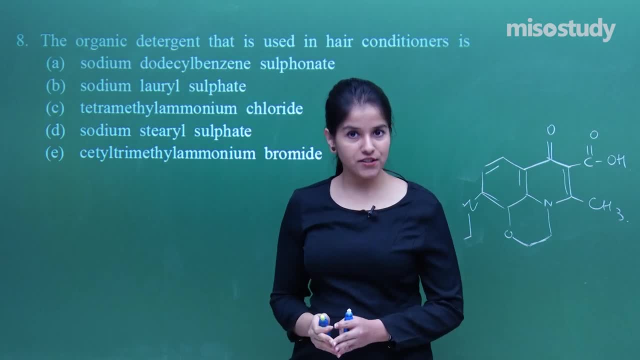 So, as we have read already in the section of detergents- those detergents which are slightly expensive- they have got germicidal properties. I hope you all are able to recall it. What is it So? yes, we have discussed. this under the category of cationic detergents. So, out of all, what is the cationic detergent that is used in the hair conditioners? It is cetyltrimethylammonium bromide. So that is the cationic. 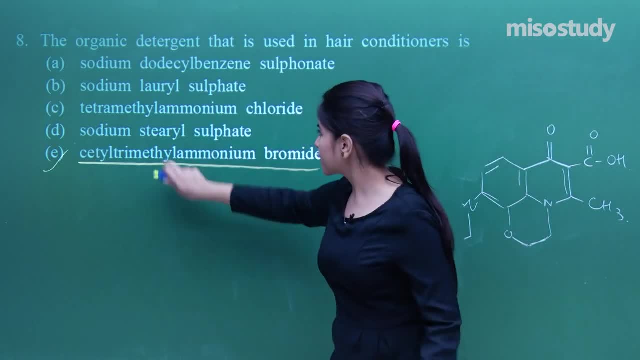 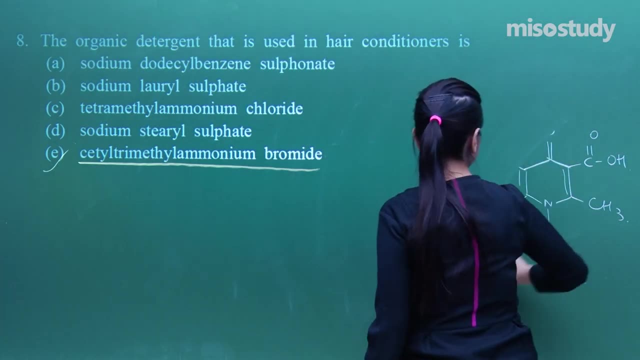 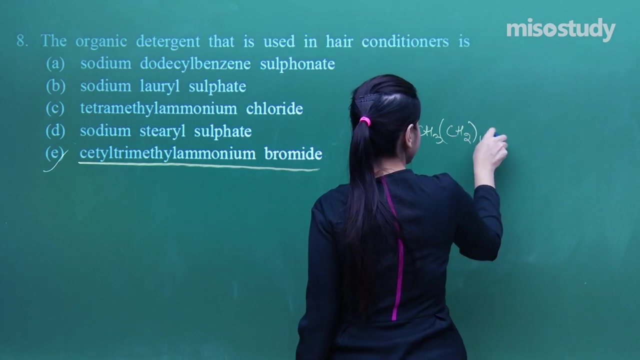 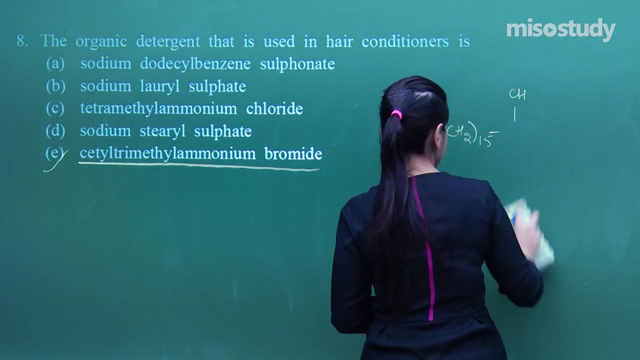 detergent that we have discussed. Do not get confused between tetramethylammonium chloride. it is not the option, So let us just draw the structure here. The structure is: it would be a nitrogen here, So it would be a nitrogen attached with. 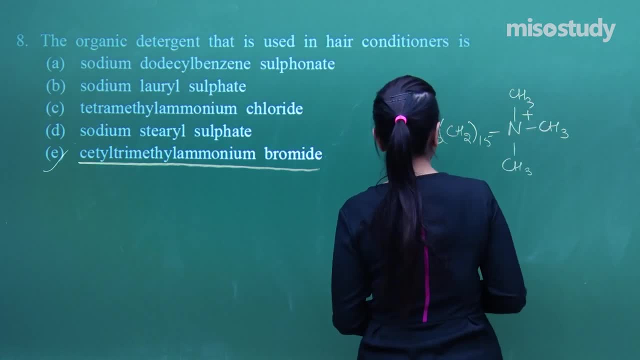 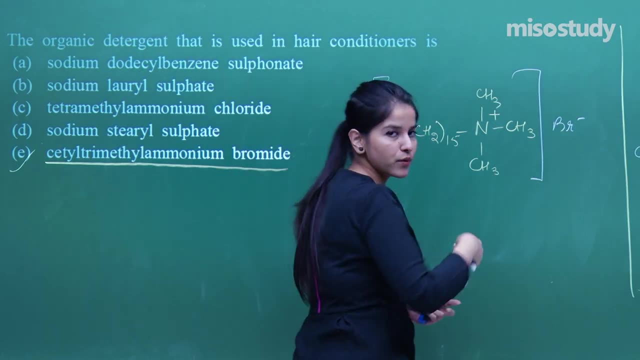 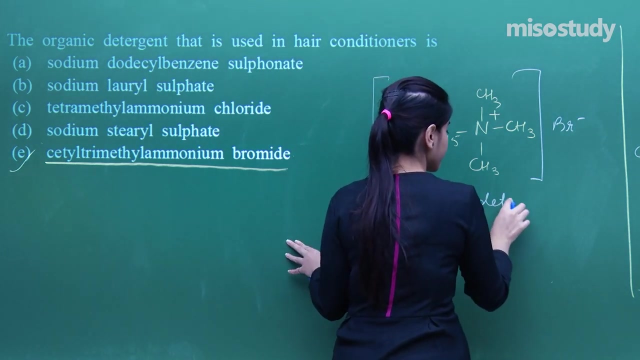 three methyls and a counter ion that is bromide here in this case. So this is the cationic part, is the bigger one. that means it is cationic detergent. So that is cationic detergent. So I hope everybody is clear. 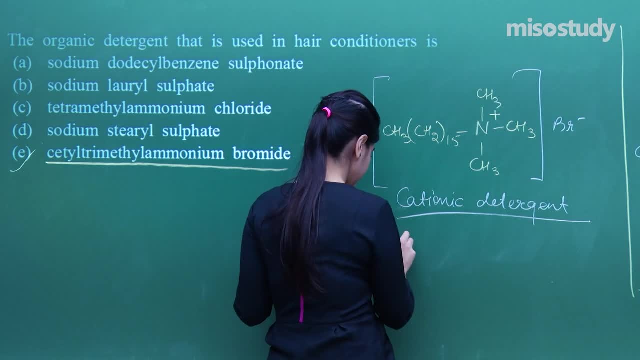 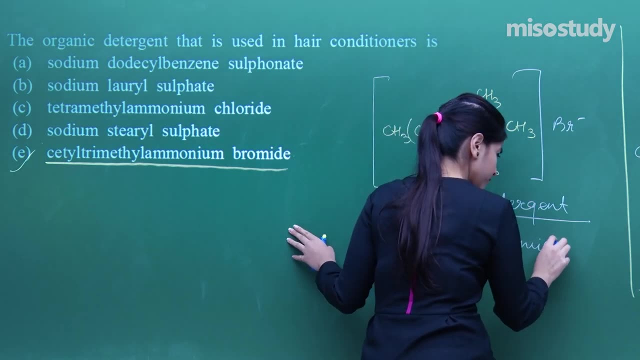 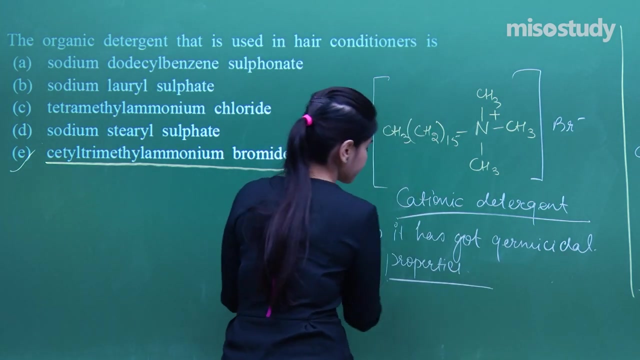 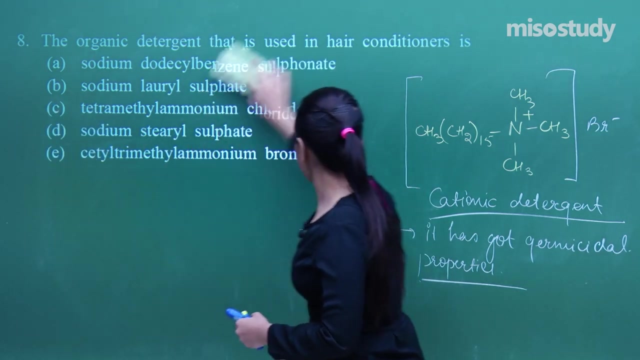 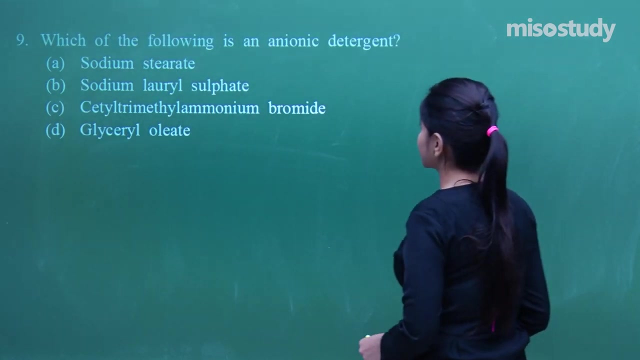 with the fact, and also it has got germicidal properties. I hope everybody has copied it down. Now let's move on to the second last question, that what we have here, Which of the following is an anionic detergent, Now comes up, the turn of anionic. 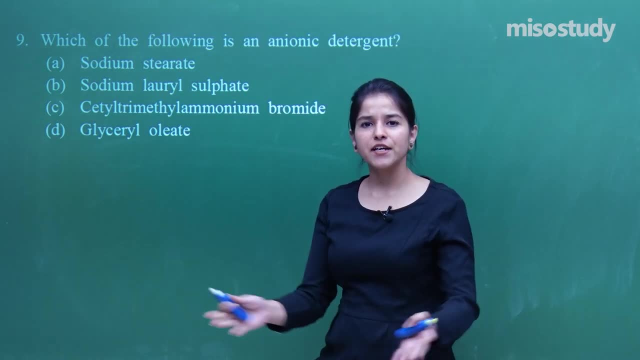 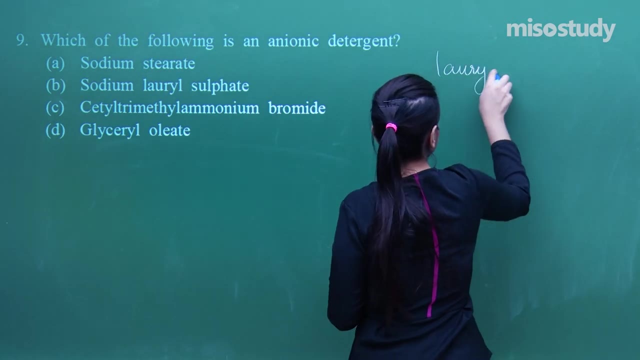 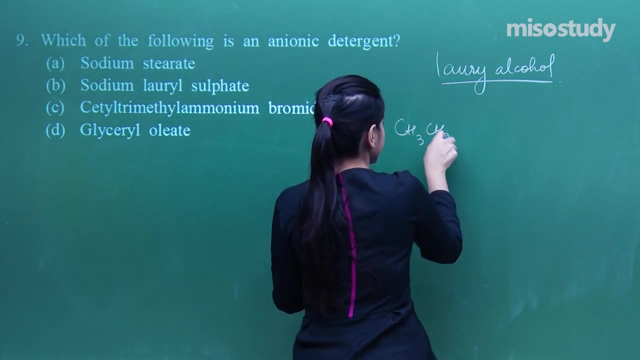 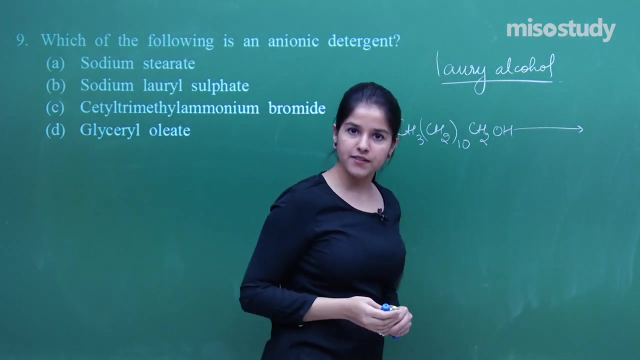 detergent. So what is an anionic detergent, Having the anion part that is bigger. So over here, in this case, we take up the laurel alcohol. So what is the laurel alcohol? it is this, and what do we do? is we firstly sulfonate it? we firstly 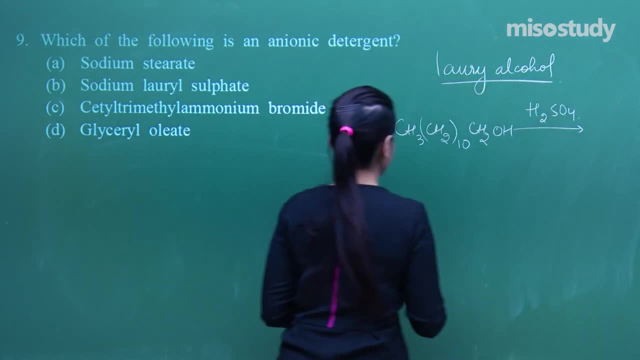 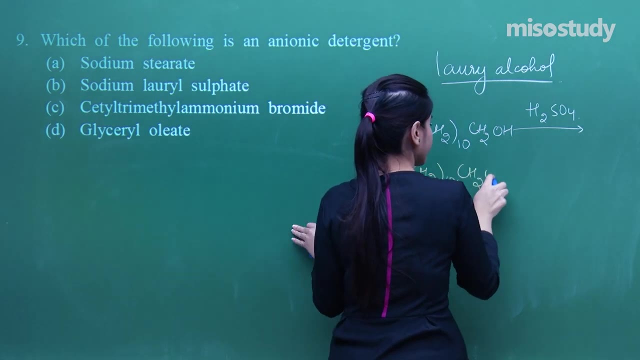 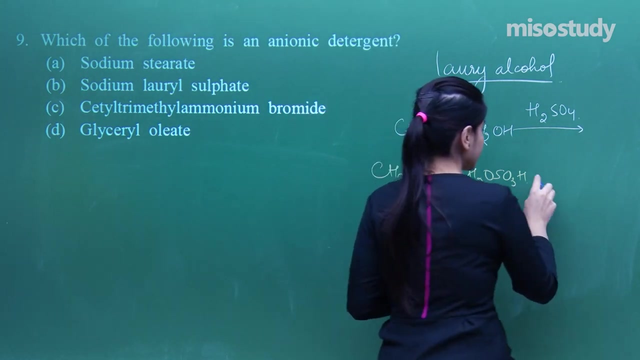 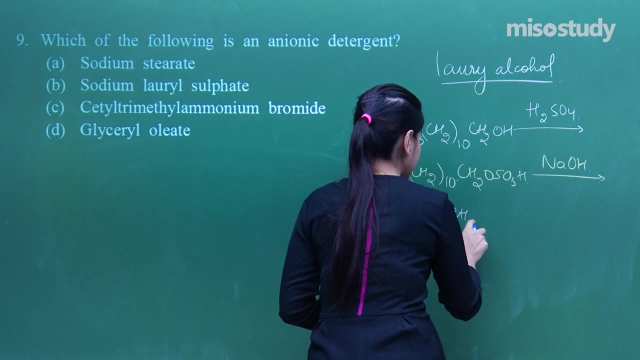 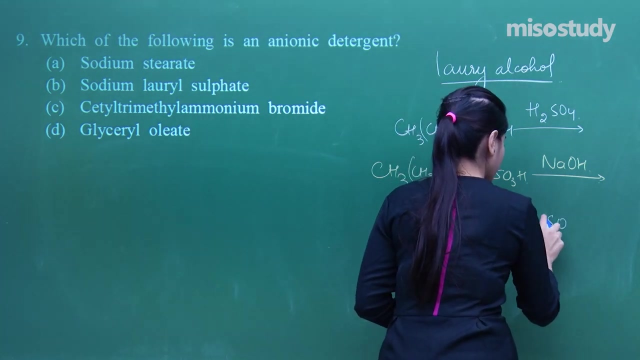 sulfonate it by sulfonation process. we get, and then we try to make it a salt and convert it into what? by making it react with the base, we try to convert it into a salt that is an anionic detergent, oso3 negative, na positive. so if you see, 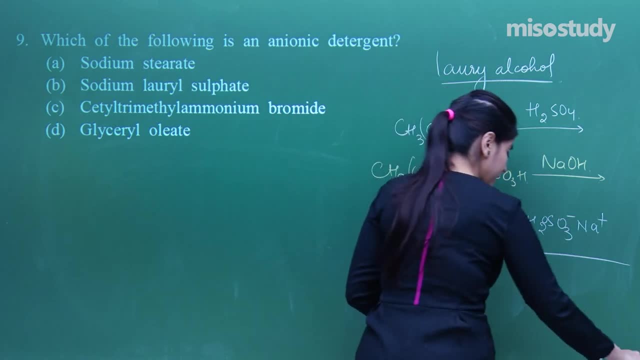 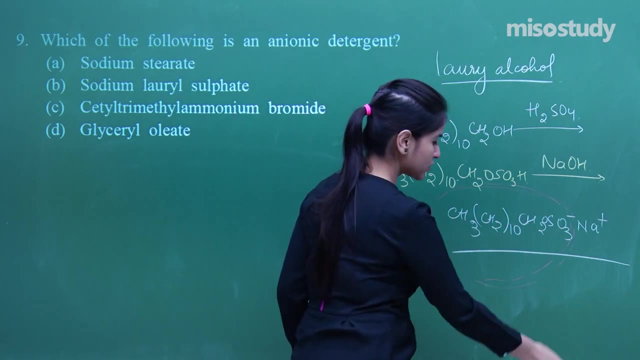 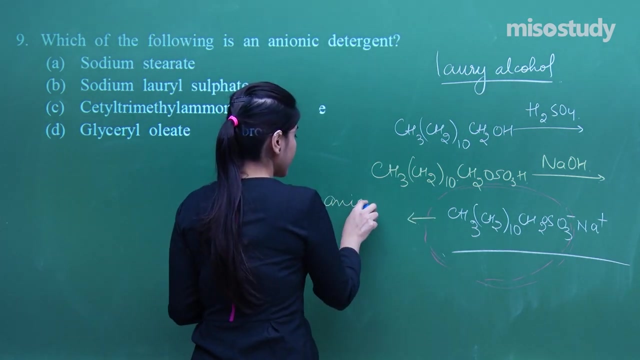 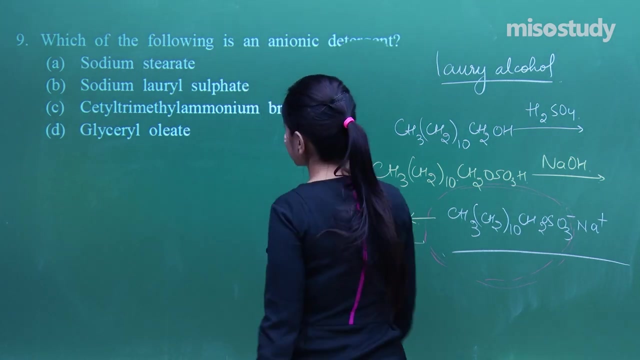 over here the anion part is the bigger one. so if you see over here there is the anion part and that is the biggest one out of the two. that means this is nothing but the anionic detergent. so that is anionic detergent and that is what sodium lauryl. 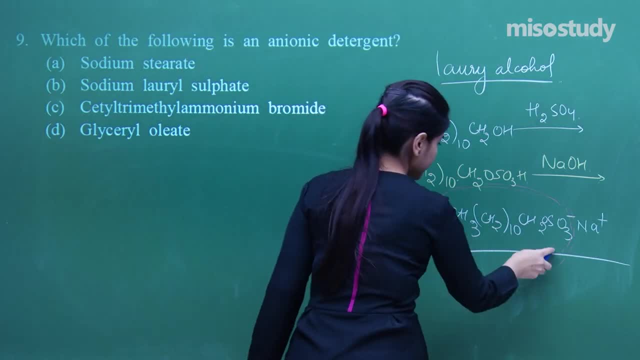 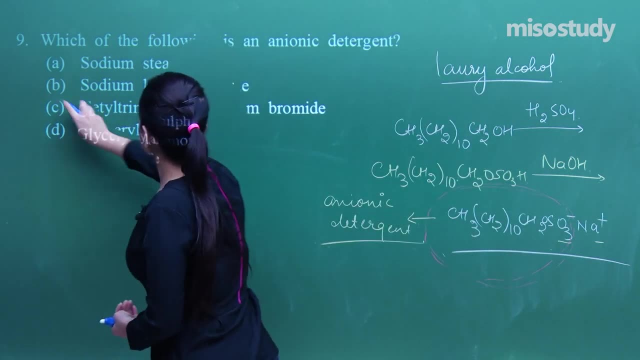 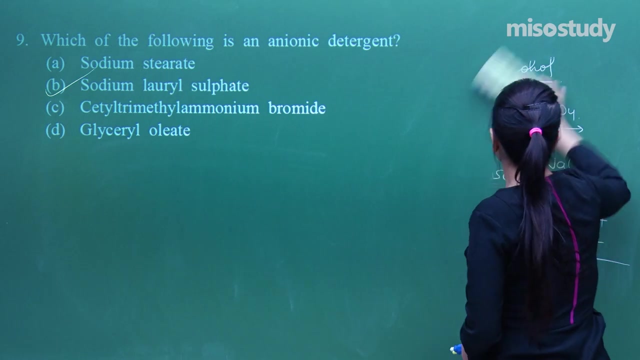 sulfate. so that is the answer. this is the laurel, this is sulfate and this is sodium, so that is how they are naming the compound, so it is sodium. lauryl sulfate is the answer. i hope everybody has got it. now move on to the very last question. what do we have? the 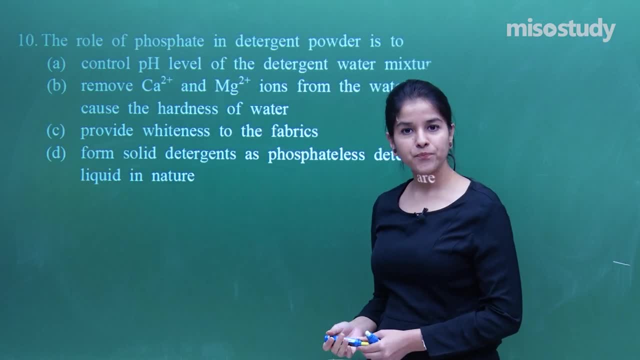 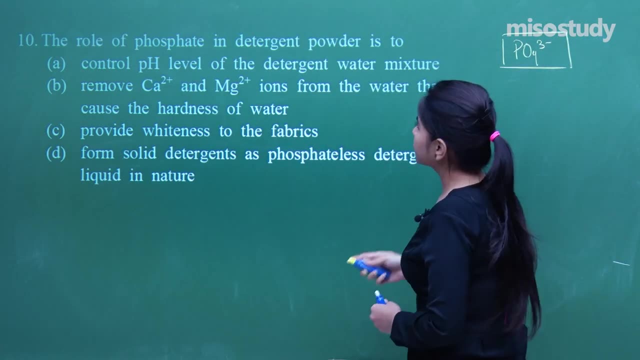 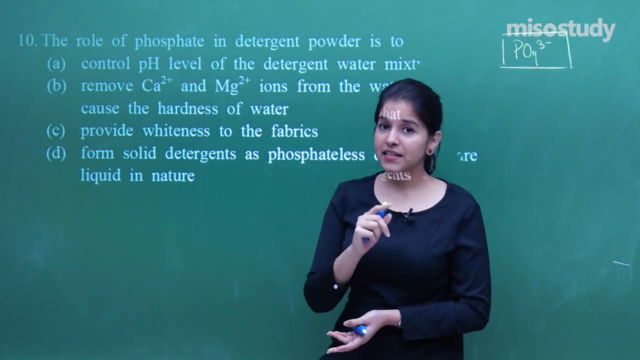 role of phosphate in detergent powder. so what is the role of phosphate? we add IU ions. what is the role of these phosphates? why detergent is not having any kind of an interaction with the hard water? That is the answer over here and it is hidden in the options. So it controls the 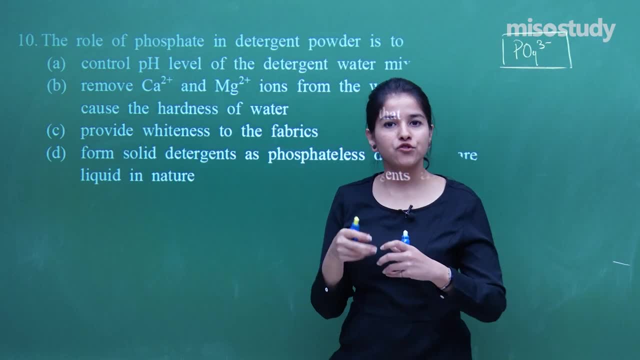 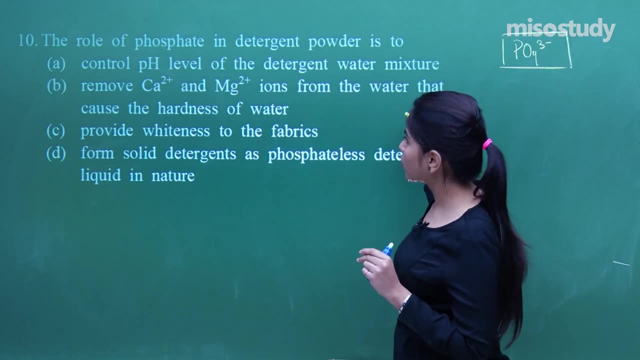 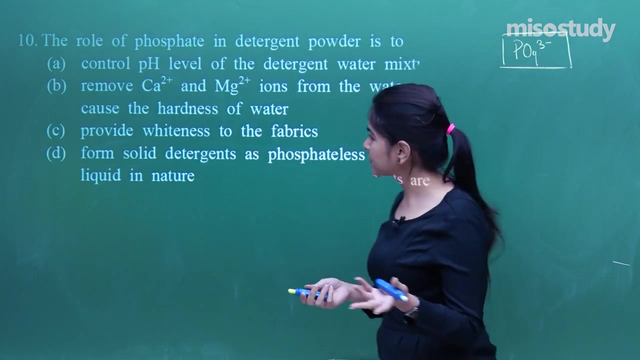 pH level? I don't think so, because hard water does not require any kind of a pH shifting, pH adjustment: Remove calcium and magnesium ions from the water that cause the hardness. It may be a possibility. Provide whiteness to the fabrics. That is not a point, It's a bizarre. 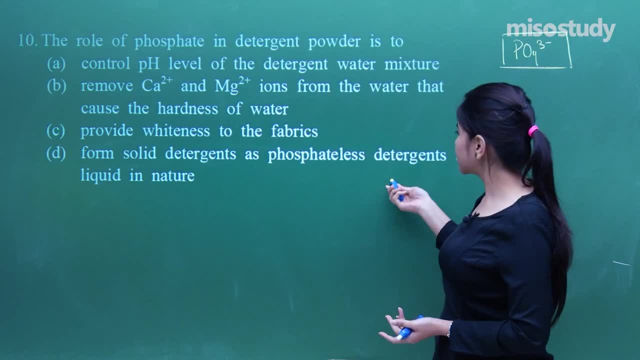 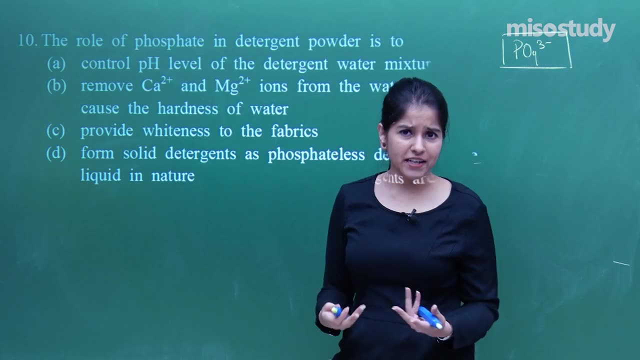 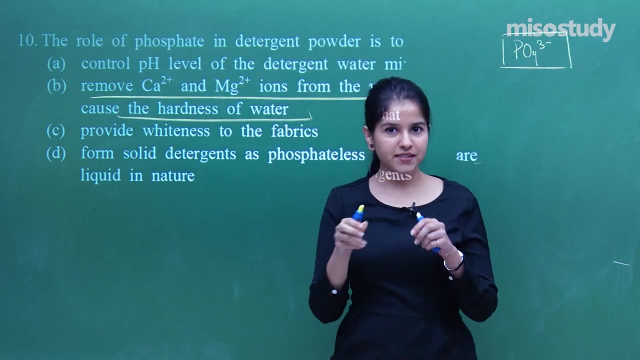 point: completely Form solid detergents, as phosphate lets less. detergents are liquid in nature, So that is also not a relevant point. I just find this point as relevant. So basically what happens is: there is hard water, It has got calcium. 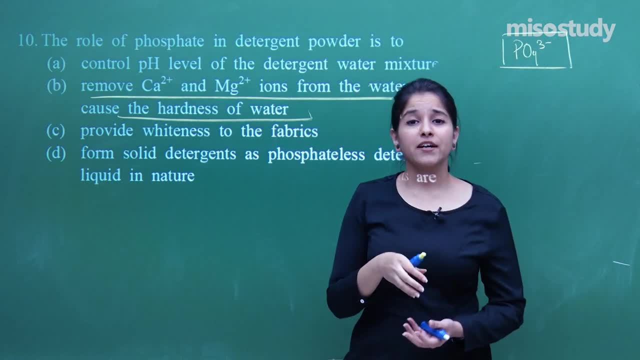 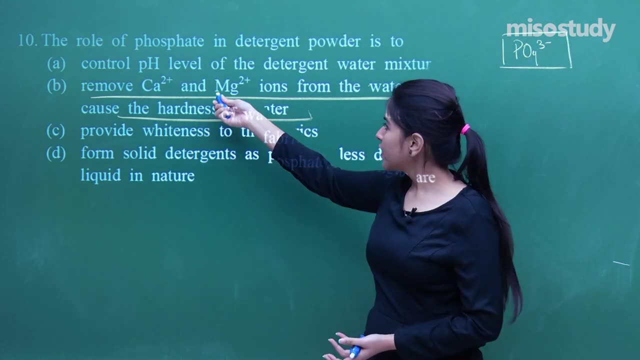 and magnesium ions. So that is why soaps- whenever we add soaps in the hard water, it forms scum, All the ions of the soap. they reacted with the what With calcium and magnesium and instead of producing the froth, they form precipitate and that. 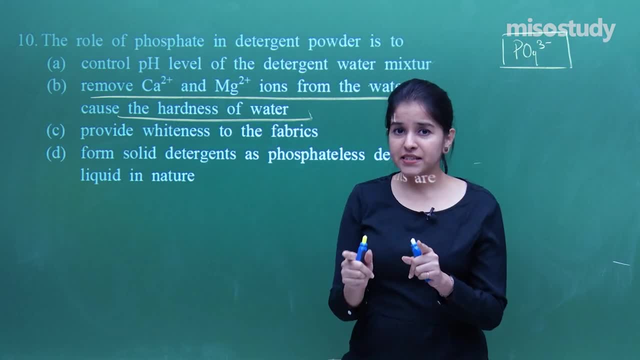 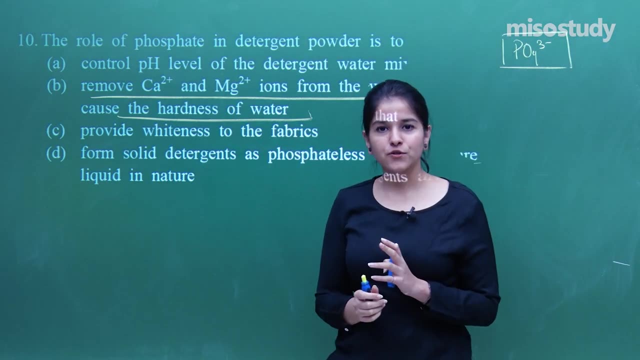 precipitate is known as scum, But this scenario is not in the case of detergents. Why? Because detergents, they are actually very good in hard water also and they produce a lot of froth. So what is happening in the detergents is they have 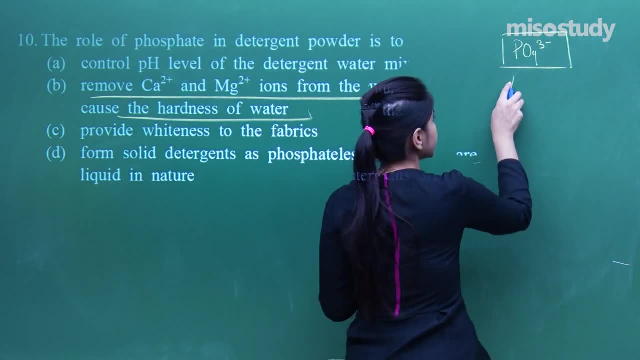 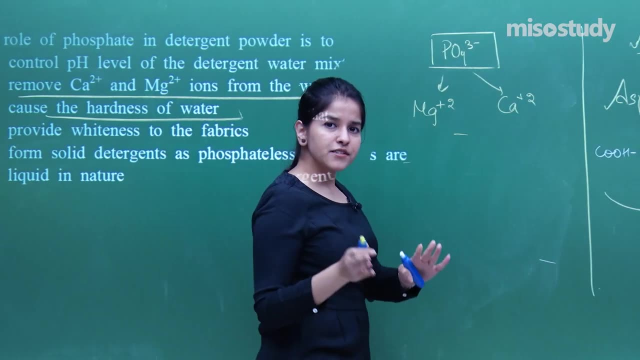 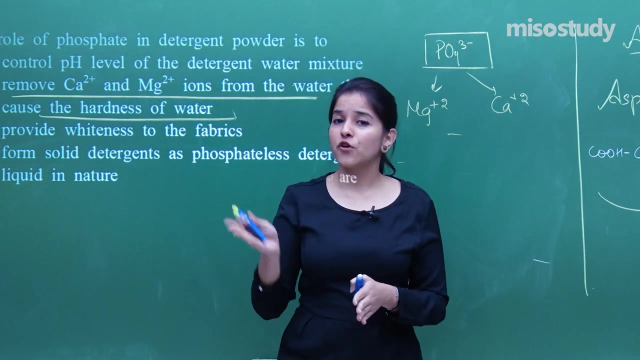 got phosphate ions into them and these phosphate ions they react with magnesium and calcium ions and by reacting these magnesium and calcium ions they are keeping these ions aside. Then these ions do not create any hindrance in the froth formation process. So that is what 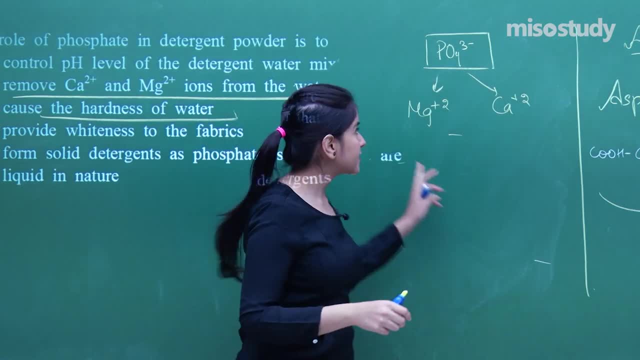 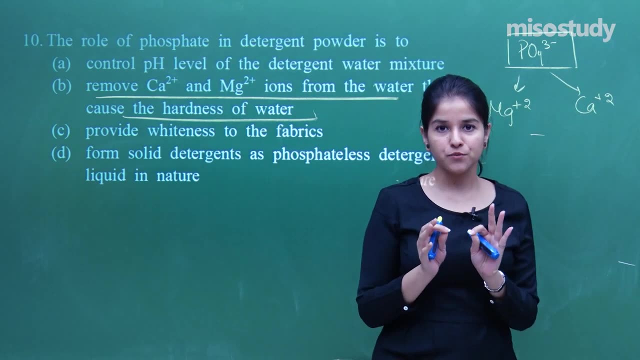 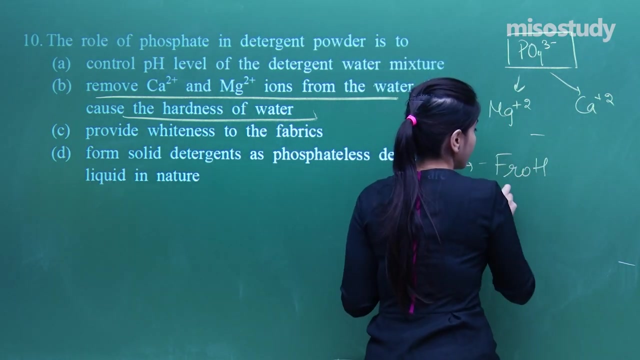 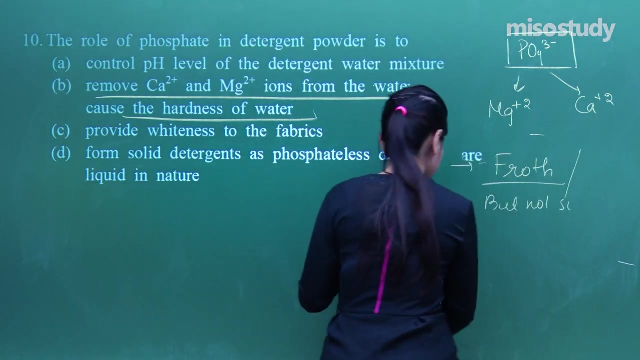 we have here. So I hope everybody is clear with the concept. There is the reaction of the phosphate with these ions, resulting in no hindrance in the froth formation process. or we can say froth but not scum, No scum formation. I can write over here. 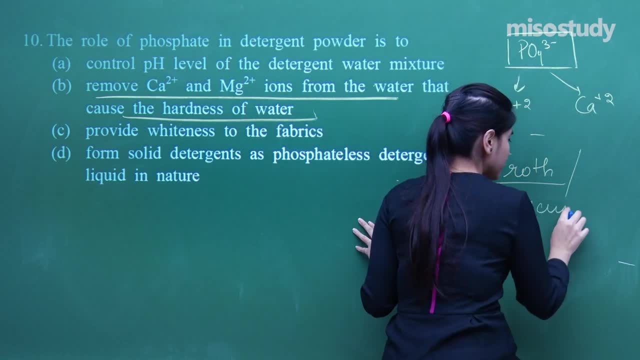 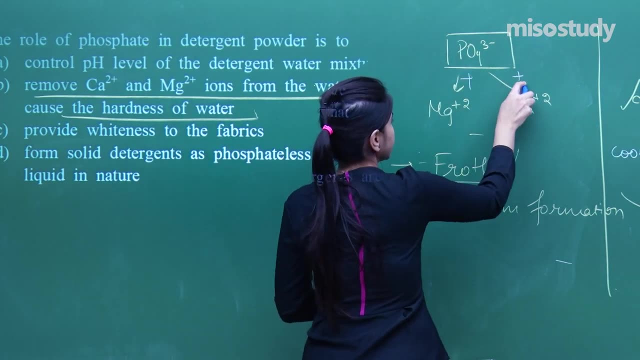 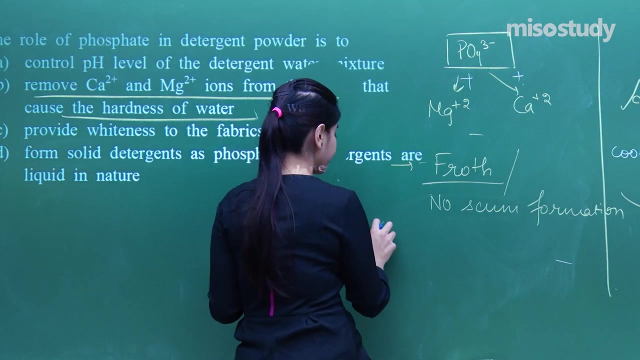 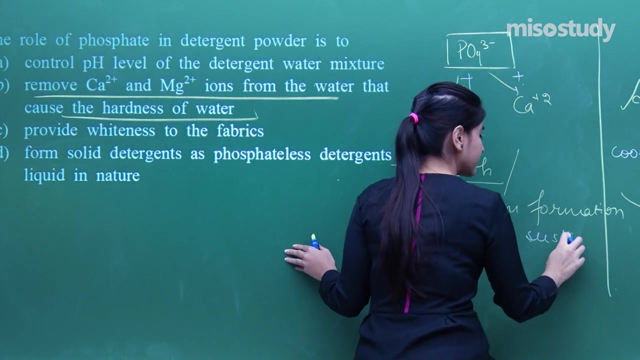 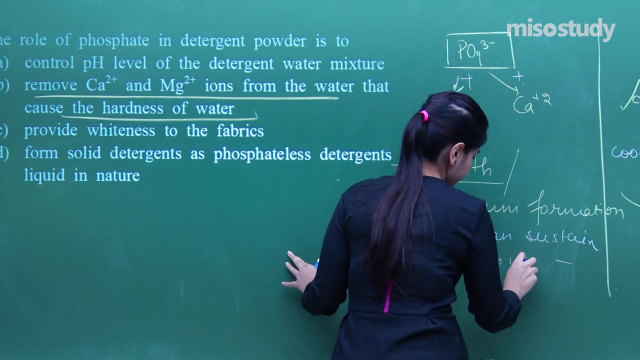 No scum formation due to this very reaction. This is the reaction that is happening in the case of detergents. That is why the detergents are also good in case of can sustain hard water as well. Ok, I hope everybody is clear with the. 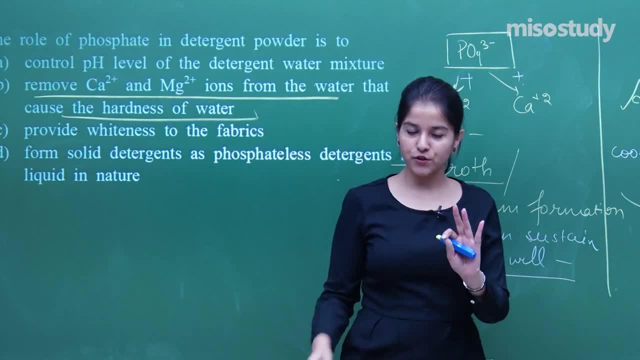 concept. Now I would like to ask you a question. So just take out your pens, if you haven't, and a paper. You need to actually write down the structural formula for cimetidine. What is cimetidine? We have just discussed That. 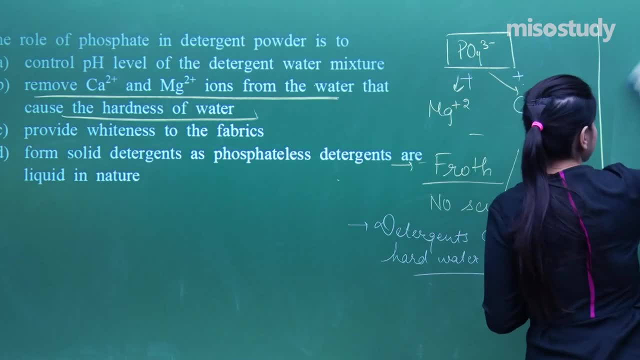 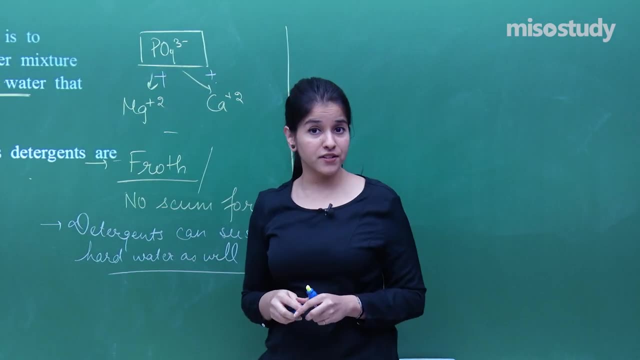 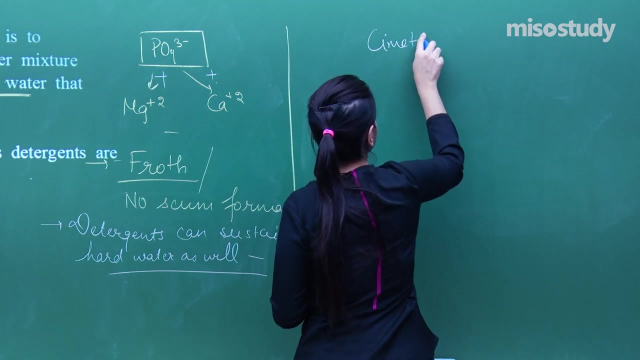 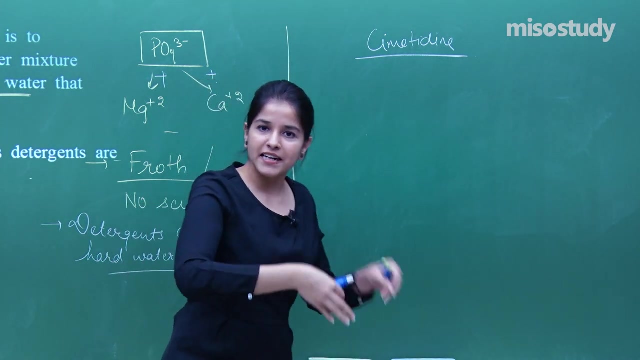 is a ranitidine. Sorry, that is just like a ranitidine, it is antacid. So what is the structure for cimetidine or tegumet that we have discussed? So the structure is it contains histidine. Yes, that is. 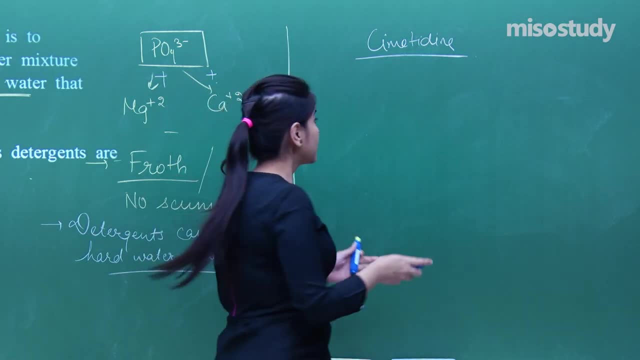 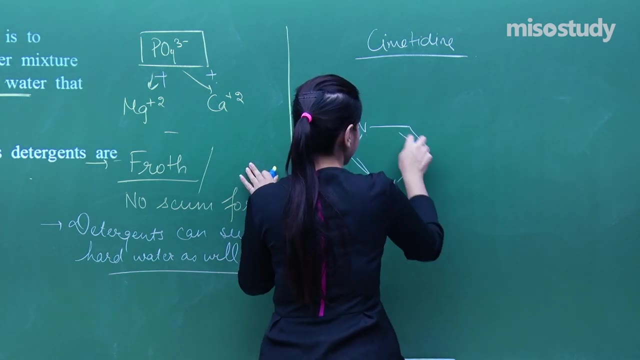 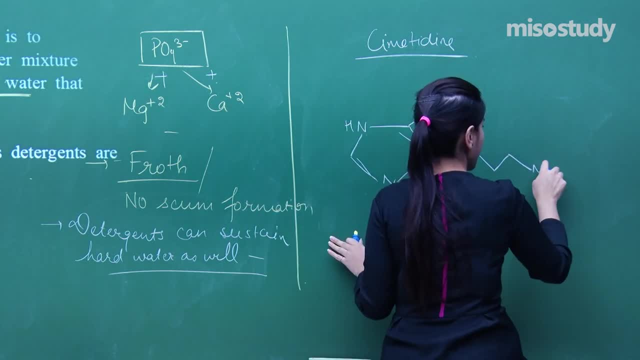 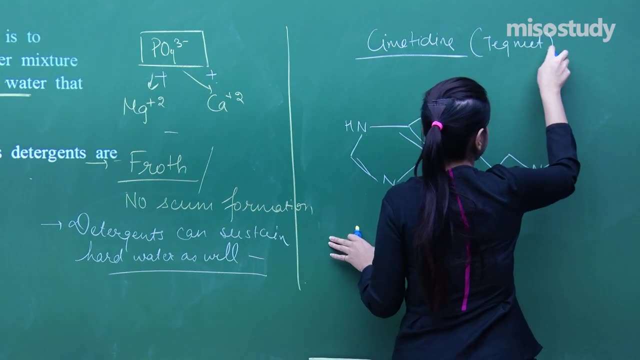 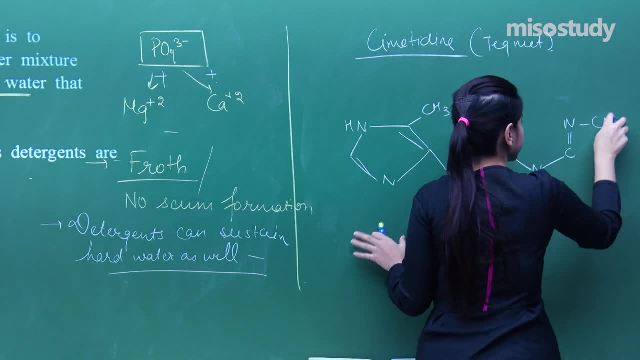 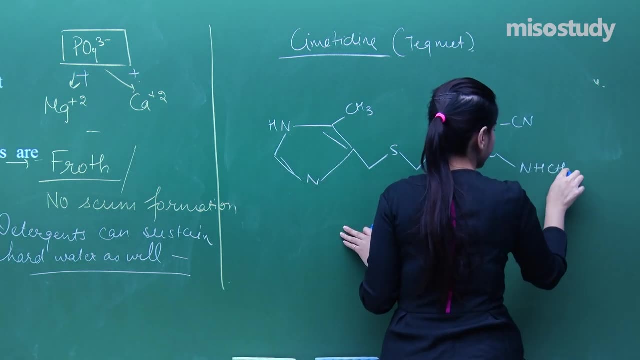 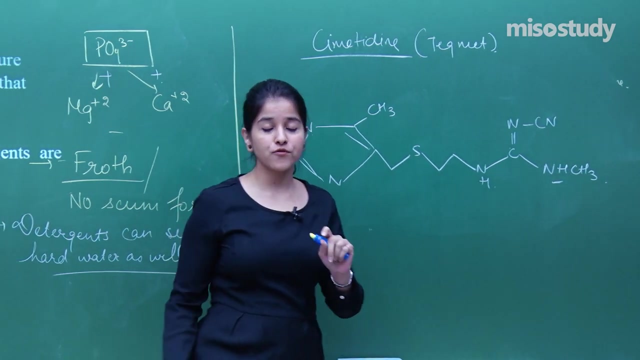 It would be. and what else do we to have Here? we have…. I said that before You need Cervical powder, So that is what Cimetidine is really useful is. you need to have a proper structurization of all the kinds of